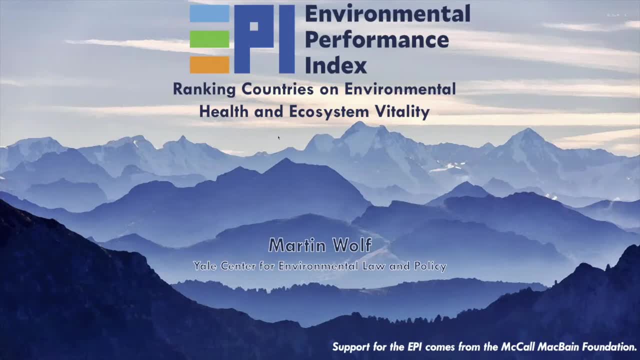 I'm actually really excited to be here to present our work on the Environmental Performance Index to you and to all of our wonderful colleagues and collaborators at the Institute for Ocean Science, for Oceans and Fisheries. So our work on the Environmental Performance Index uses data driven analyses to quantify environmental health and then ecosystem vitality. 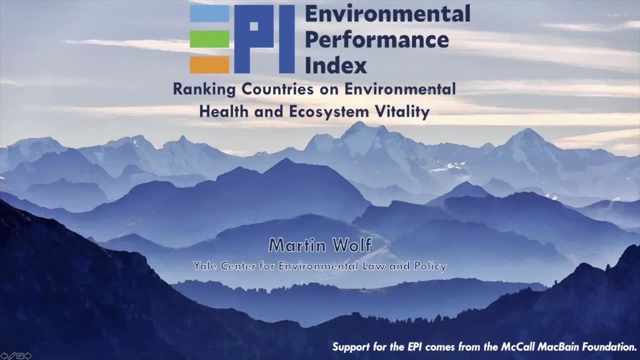 And we'll get to how we define these two overarching goals- Environmental health and ecosystem vitality- a little bit later on in the presentation. But I guess I'd just like to start by saying at the end: I hope I've convinced you that the EPI isn't just a report that we published, but rather it can be a tool that countries and policymakers within countries around the world can use to both track environmental trends within their borders and also identify policies that can improve their sustainability. 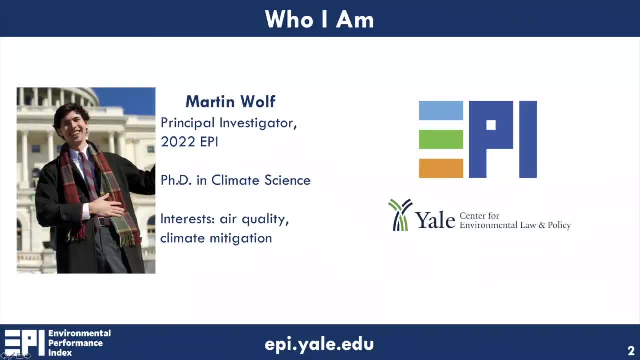 Thank you. So Deng already gave a great introduction, But just to help you put a face to the voice, I'm Martin, And what I am is the principal investigator of the 2022 Environmental Performance Index. So my background, as Deng said, is in climate science and atmospheric chemistry. 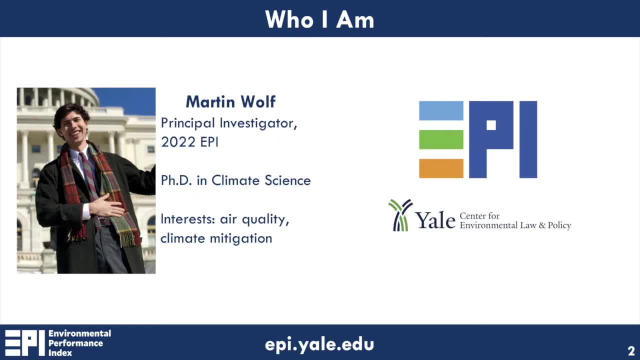 And while I was in grad school I was really fortunate to work with many Canadian colleagues, including Alan Burcham, who is a professor of chemistry at the University of British Columbia, on sea spray aerosol emissions. So the ocean lies close to my heart. 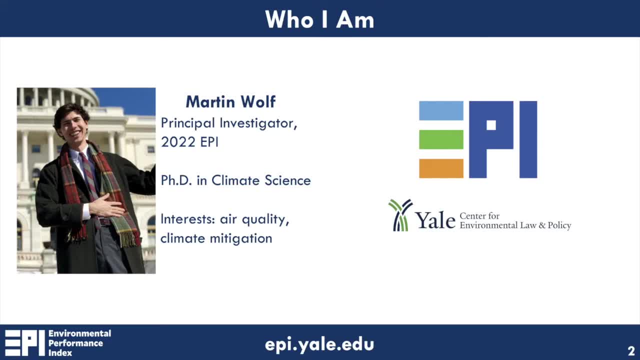 So if I'm given a label, it's atmospheric chemist And, as Deng mentioned, I'm now a postdoc in charge of the Environmental Performance Index, which is housed at the Yale Center for Environmental Law and Policy, which is a center that's split between Yale Law School and the Yale School of the Environment. 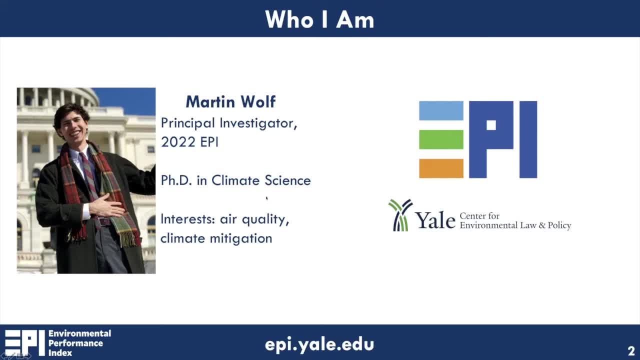 So I know that there's a Q&A session after the talk for Iowa students only, But if any of the students have any questions during that time, not only about the science that I'll try and present today, but also about students, Thank you. 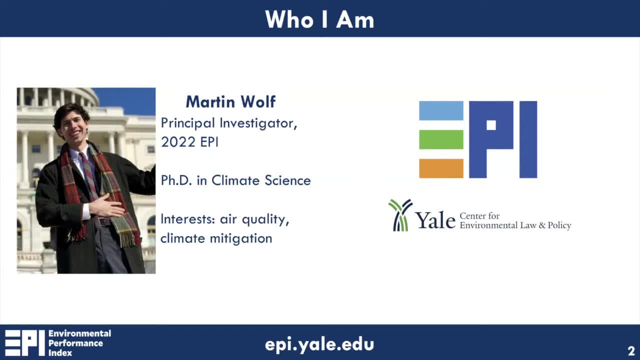 I'm Deng And I think this is an important discussion today, but also about straddling the traditional great chasm between science and policy. Feel free to ask me about my experiences. Happy to talk about my time in Washington DC before my postdoc, et cetera. 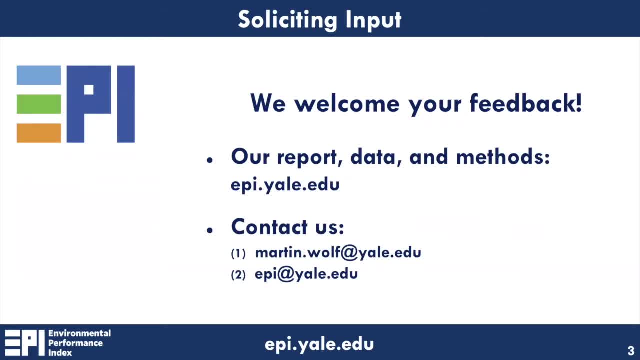 So I hope that this will be a kind of fun and informative discussion. So there's anything that's incredibly unclear while I'm talking, Feel free to stop and interrupt me for questions after the presentation as well. So, as always, we're eager to solicit your feedback. 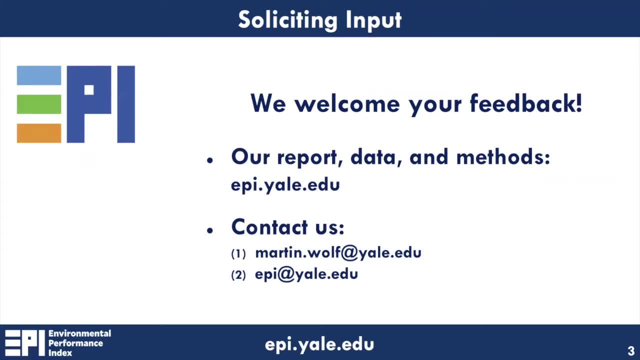 One of our goals of the EPI is to kind of keep it fresh and relevant by polling experts in environmental science like you on new ideas and also suggestions to improve our data sources and our methodologies and the like. So please feel free to contact me later or tell me now We'd. 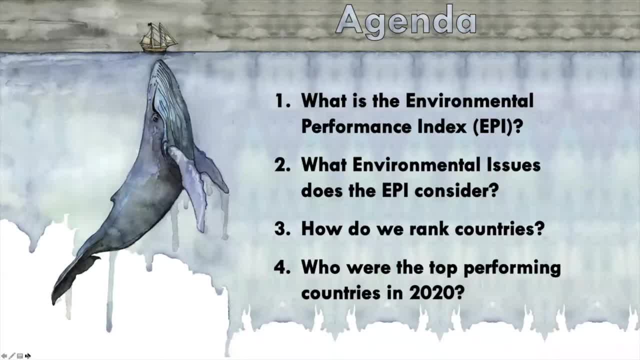 love to hear your feedback. Okay, so what's lurking beneath the surface of the seminar today, you might ask. Sorry for the visual pun, but first we'll talk about what the EPI actually is, what the Environmental Performance Index actually is, and also what it's good for. 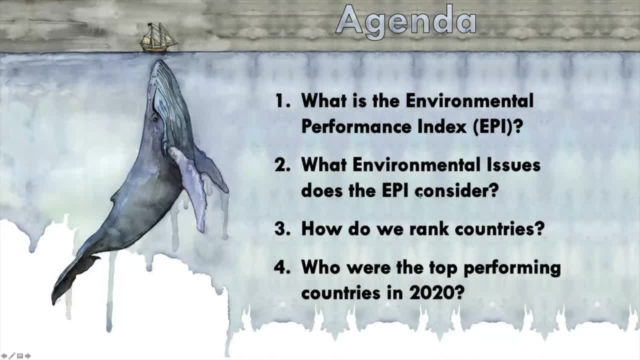 So we'll talk about what environmental issues the EPI considers and we'll spend a particular amount of time on the marine issues that we check, And then we'll also talk briefly about what environmental issues the EPI considers, and then we'll also talk briefly. 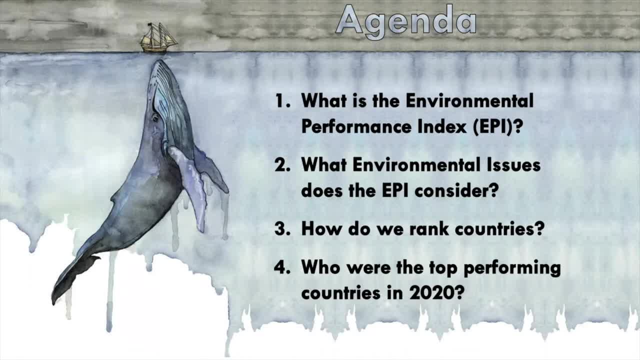 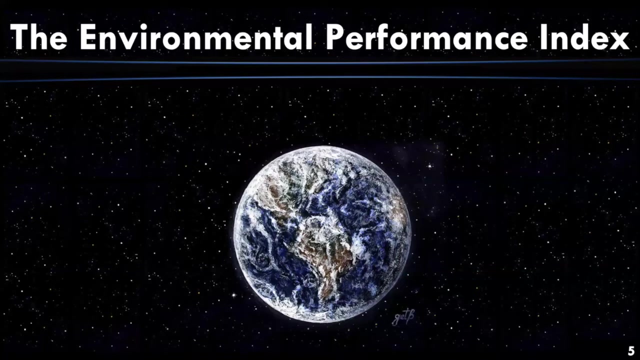 about how we derive our results, so how we use data in order to rank countries, before finally getting to the entree of the agenda, which is the results. so who were the top performing countries in the 2020 analysis for various environmental issues? So we can dive right into the Environmental 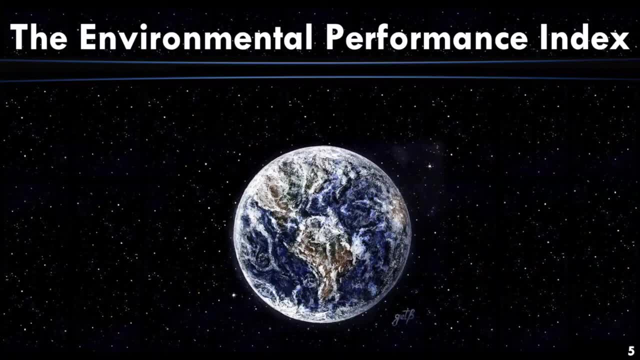 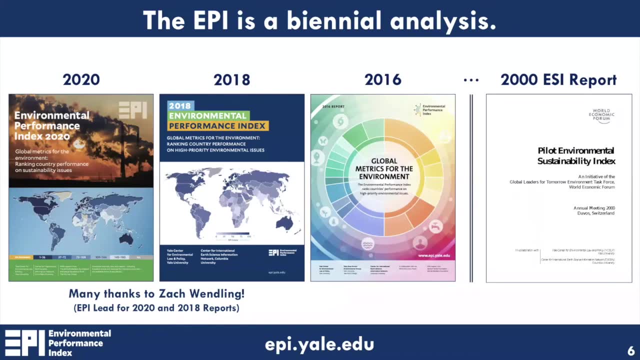 Performance Index. I said at the very beginning that ostensibly, the Environmental Performance Index is a report And at face value it's true. The EPI, or Environmental Performance Index, is a report that's now in its 20th year, or 10th iteration, because it's a biannual. 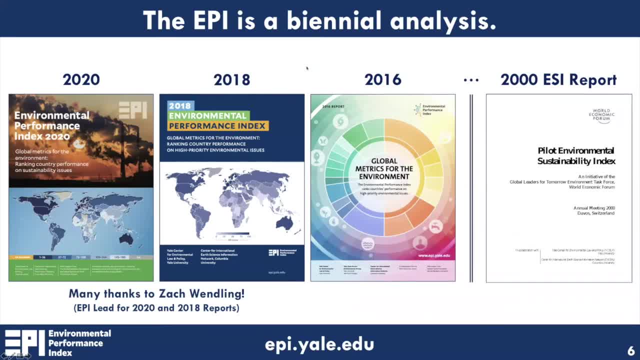 report And over that time, it's really grown into something that we're quite proud of, especially in recent years under the leadership of my predecessor, Zach Wendling, who directed the 2018 and 2020 reports, as well as its predecessors before them. 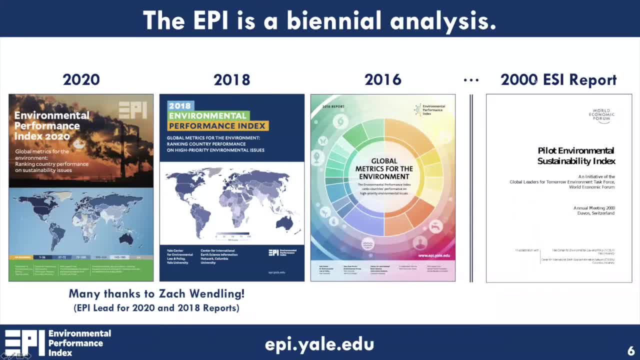 So if you trace the EPI back to its roots, you can see that it originally started as something called the Environmental Sustainability Index or ESI, which was started all the way back in the year 2000.. Now the current Environmental Performance Index, EPI, differs from the original. 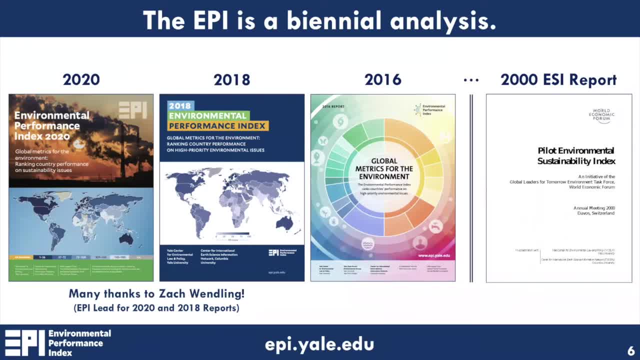 ESI Environmental Sustainability Index, And then we place more emphasis on really environmental outcomes. So measure, in other words measuring and tracking trends and environmental issues rather than sustainability issues more broadly. So since the year 2000, the Sustainable Development Goals 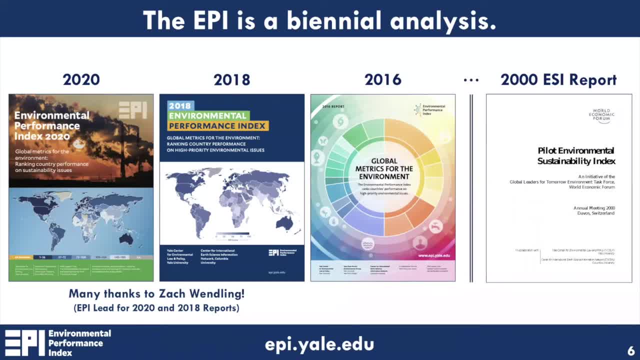 superseded the Millennium Development Goals And there's been a broader emphasis on sustainability outside the realm of just environmental science and environmental issues, which are incredibly important, But we specialize in measuring and tracking trends specifically in environmental issues rather than the sustainability issues more broadly. So the 2020 Environmental Performance. 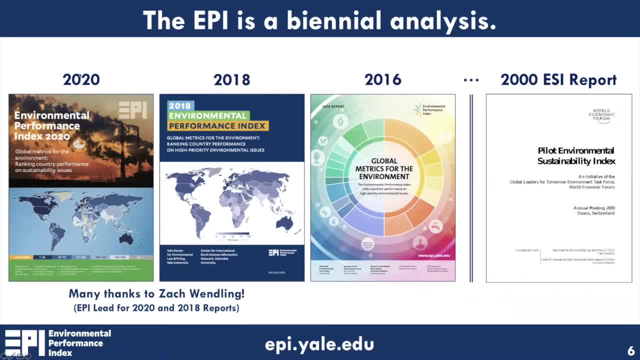 Index report. it's the most analysis that we've done to date in terms of the number of countries covered and also the kinds of issues and the number of issues that we examine, And it also uses just the latest global data sets, not only to check the environmental trends over time, but 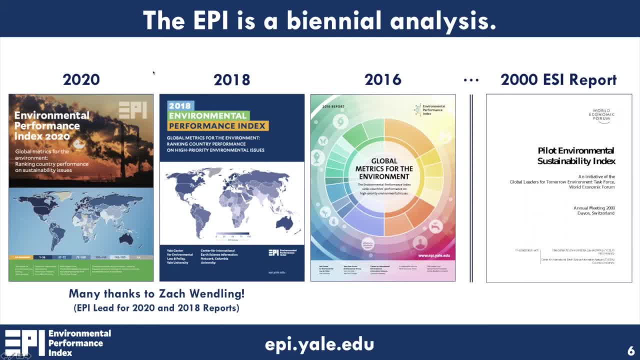 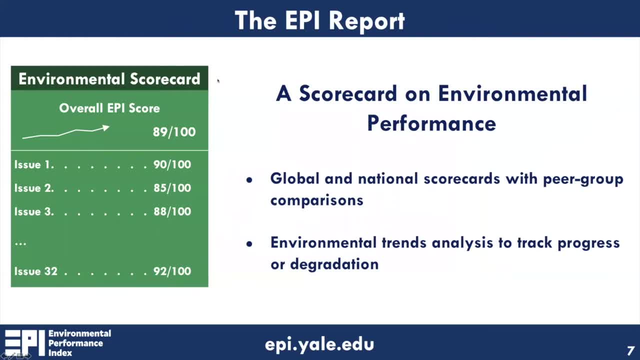 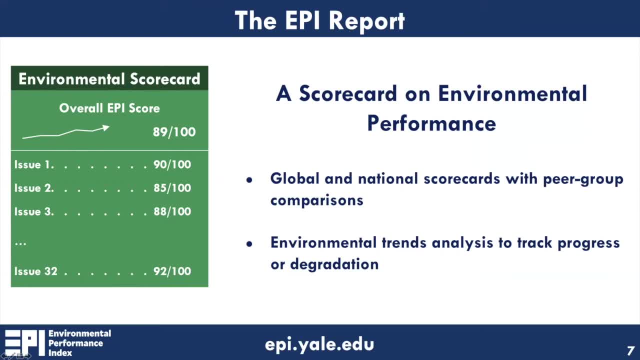 or EPI reports. So, as we'll see a little bit later on in the presentation, we offer both global scorecards- so how is the world as a whole doing? As well as national scorecards and regional scorecards with plenty of 960 selector total scores, And they're designed to simplify general 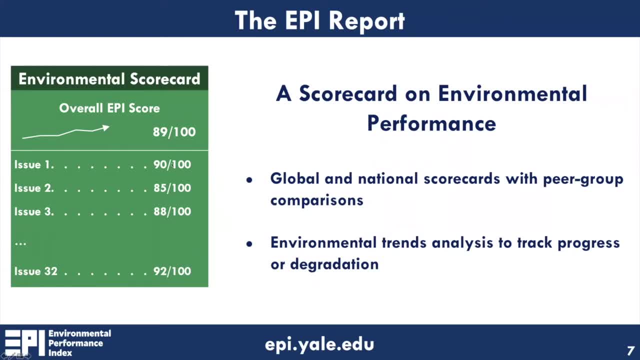 of information that countries can really use to compare their own performance against their peers and really get down into the weeds if they're interested in specific issues. So, importantly speaking of specific issues, we check not only environmental performance in the year that the report is released for all of these issues, but we also compute trends to check how a country's 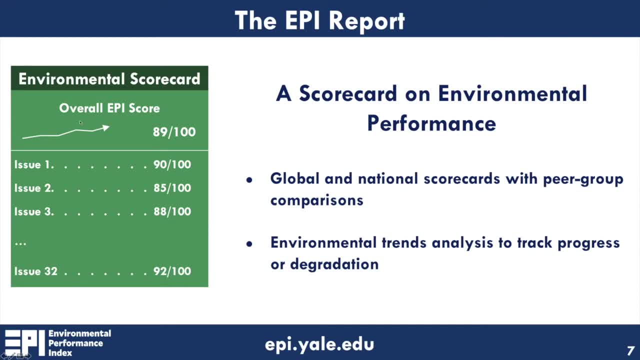 scores are really making progress or, unfortunately, in many issues, regressing in certain environmental issues over time. So in the end, what we do is we take data and various environmental issues and the 2020 report. we considered 32 different specific issues. We compute a score and a ranking. 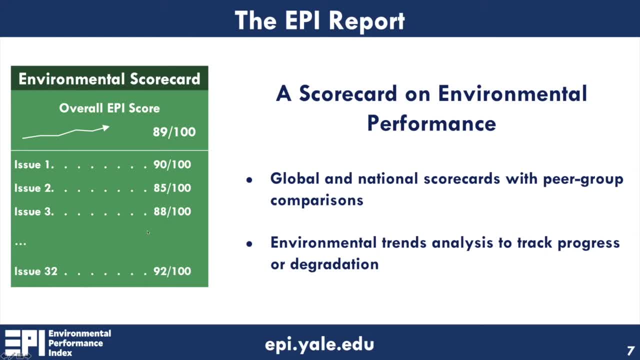 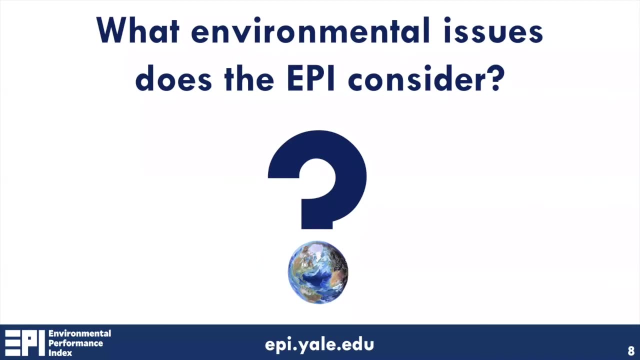 for each and then give each country a final, or really overall, environmental performance index score that reflects performance in all of these individual indicators. So you might ask: what are these actual individual indicators that we consider and really, what specific issues do they track? So, as environmental data science has grown over, 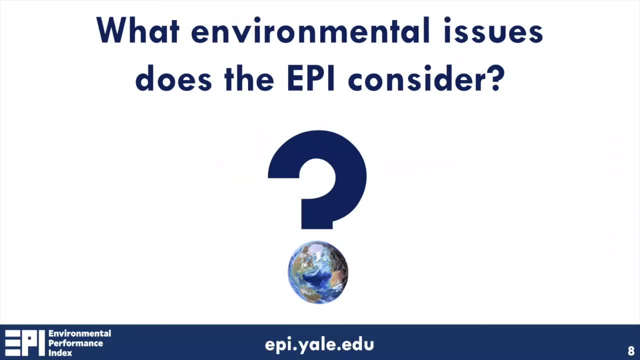 the past- really decades and even really recent years- and the data have become more thoroughly tracked and reported and global in scope and coverage. VPI has kind of really grown into something over its 20 years of existence to encompass a fairly comprehensive set of indicators that track a whole variety of different environmental issues. So let's just take a look at 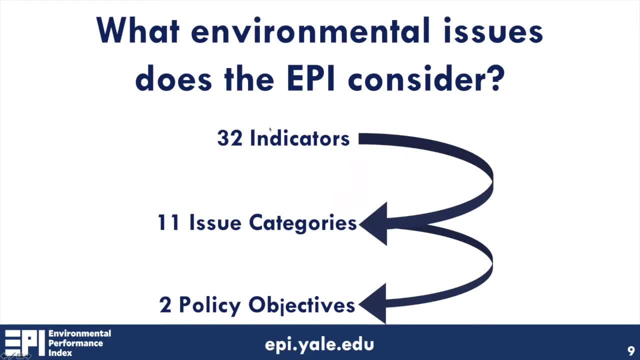 what they are. So, in more specificity, we check 32 different environmental issues that range from things like greenhouse gas emissions to water quality, to biodiversity and habitat conservation, And then we can group these 32 individual indicators into broader issue categories. We have 11 issue categories, which themselves are grouped. 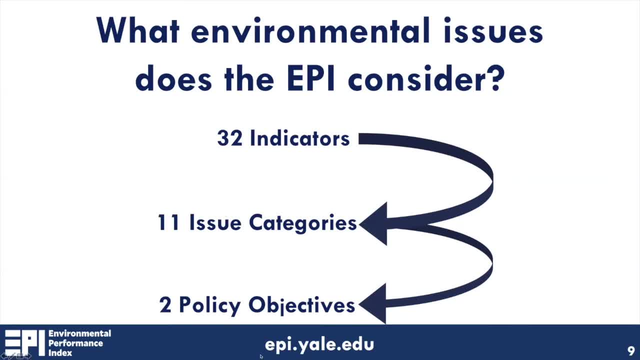 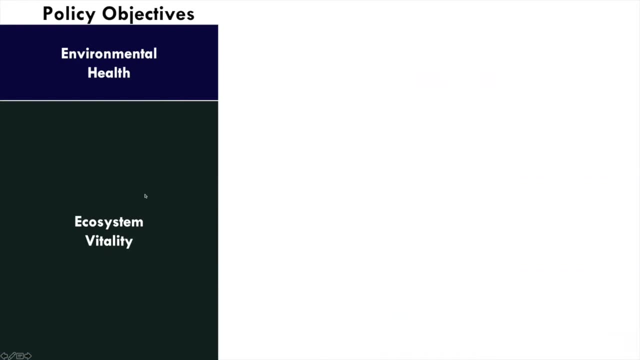 into two even broader policy objectives. So this tiered structure really provides the overall framework For the environmental performance index. So, going into all of this in even a little bit more detail, the EPI analyses have consistently tracked over its 20 years, or I can say, at least since the past. 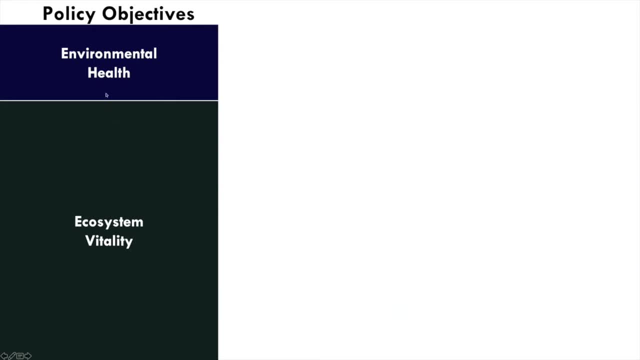 since 2006,. performance in these two broad policy objectives, which are- we hope they're- fairly simple and easy to understand. but we want an environment that keeps people healthy, which we call environmental health, And then we also want good practices. 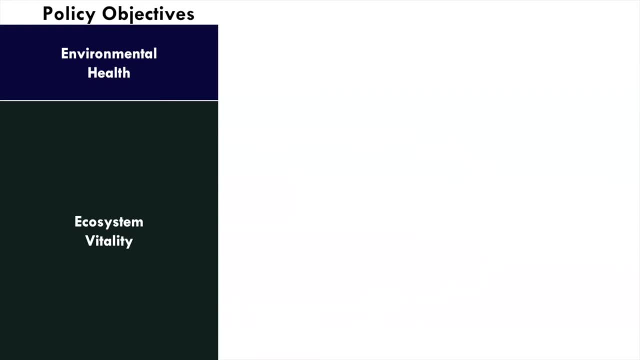 and good performance that allows nature itself to flourish, which we call ecosystem vitality. So all of the environmental issues and the indicators that we use to track the issues, we can divide all of them so that they fall under one of these two broad policy objectives. 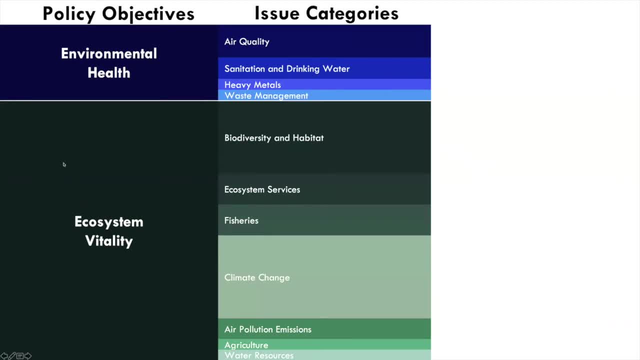 So, beneath the policy objectives, we have these 11 issue categories. At least, we had 11 in the 2020 environmental performance index. Four of these issue categories fall under environmental health and seven fall under ecosystem vitality policy objectives. So I'll briefly note that it isn't a perfect system and you could easily make arguments as 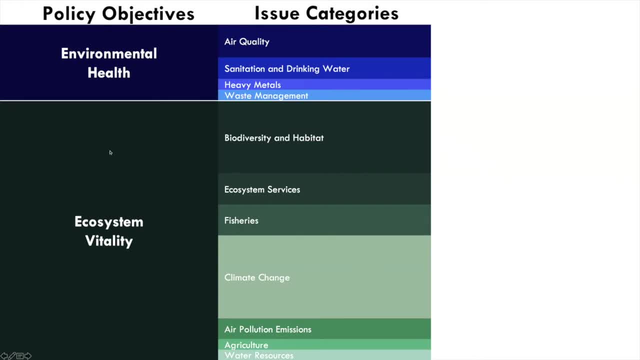 to why different issue categories should fall under both environmental health and ecosystem vitality, Like, for example, take climate change. You can certainly point out that there are public health implications of climate change, in addition to the implications that climate change has on the vitality of the ecosystem. 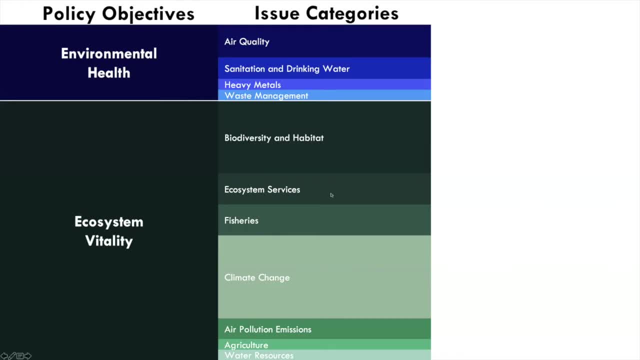 And natural processes, But we hope that it makes sense that, at the end of the day, the most important thing isn't really how we try and put labels on issues by classifying them, but rather that we're considering them and showing that countries through monitoring of their performance and trends, 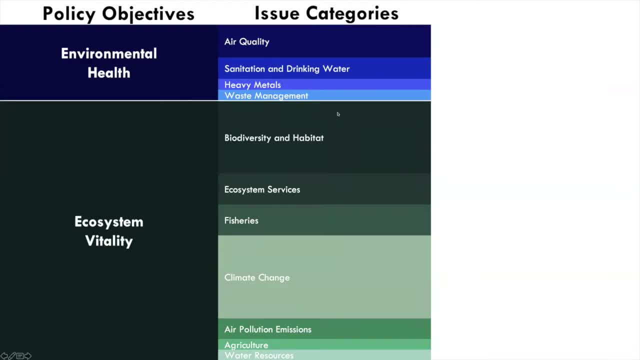 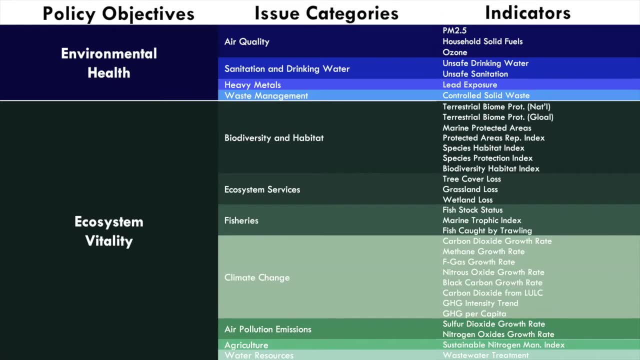 can improve their environmental performance. So, within these 11 issue categories, we finally get to the specific issues or indicators that are used to track specific issues, And you can see that. well, the list is pretty long and I won't have time to read it all today. 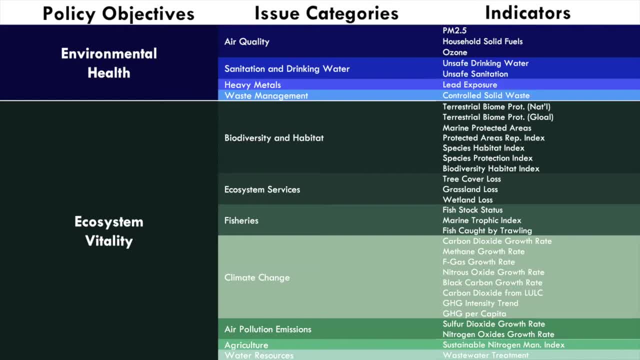 but I hope it gives you some idea of the comprehensiveness of the analysis that we do for the EPI. But we're also very curious to hear from you if you know of any other good global data sets or other important issues that we're not considering here. We're aware that there are many issues that 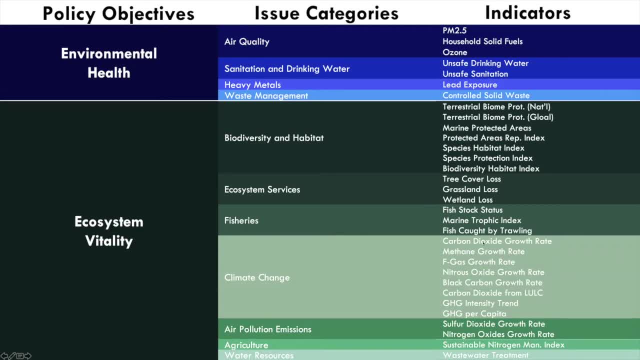 are included in this list, but the key is: is there good enough global coverage of data in order to compute scores and rankings for countries? So I don't have time to review and list off each of the 32 distinct environmental indicators in great detail, which is too bad, because I'd absolutely 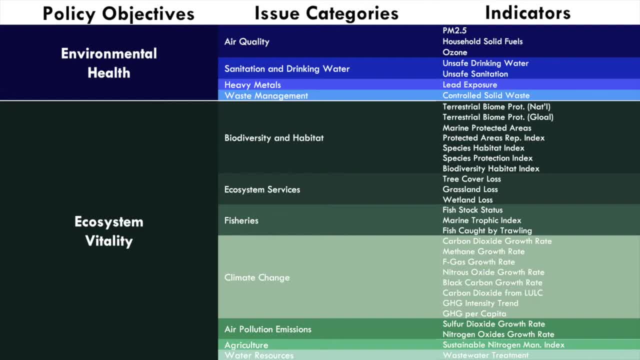 love to, but I'm guessing you have better things to do with your Fridays. So rather than just go through and read them out, I'm just going to quickly flash some pictures in front of your eyes and help you visualize and hopefully internalize some of them. So climate change. 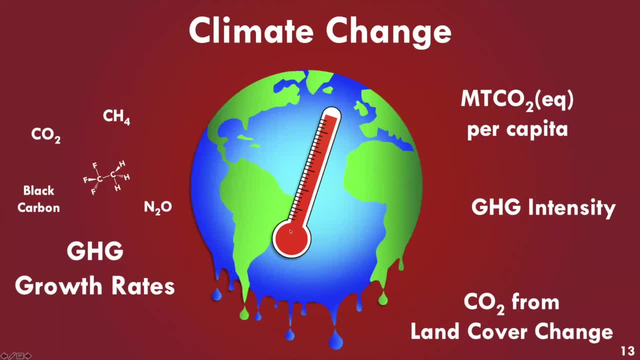 which is one of our broadest issue categories, And the individual indicators that we consider within the climate change category are the growth rates of different greenhouse gas emissions, including the usual suspects like carbon dioxide and methane and F gases. And, by the way, I've been 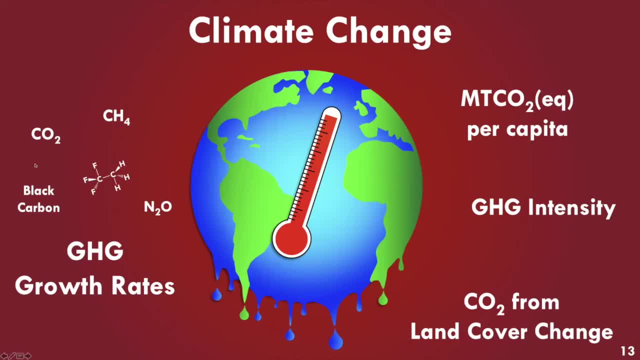 closely following Canada's efforts to phase down fluorinated refrigerant emissions, And I'm so glad to say that Congress here in the United States has finally given our environmental protection agency, EPA, the mandate to regulate HFC emissions as well. So we'll be learning a lot from our 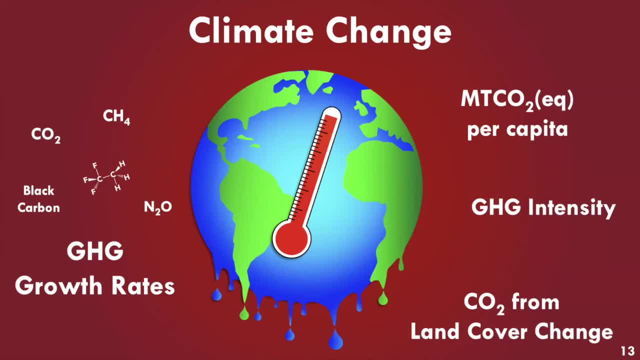 northern neighbors in that process. I'm sure We also have other indicators that provide a more- I guess you could say standardized- comparison of climate action, like greenhouse gas emissions per capita and also greenhouse gas intensity, which measures the greenhouse gas emissions per unit. 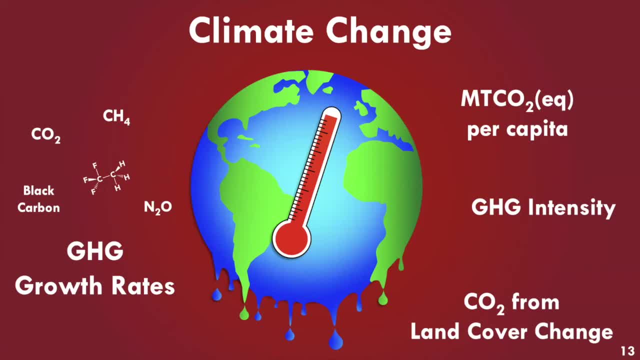 of GDP, gross domestic product, And then in the 2020,, in the 2020, API. excuse me, there was also another indicator, which was CO2 emissions from land cover change. So converting from forest to agricultural land, for example, there's a greenhouse gas emission associated with that. 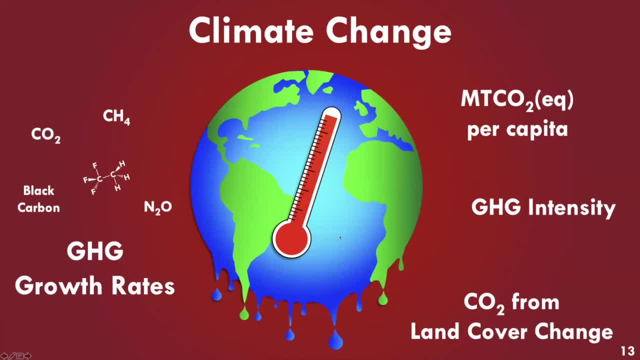 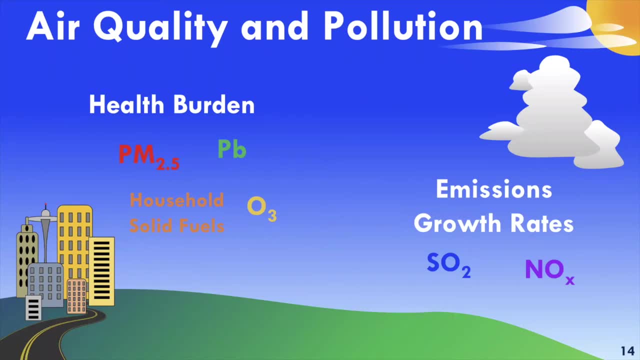 change. So we were able to account for that for the first time in this past report. So we also track air quality and air pollutants in addition to the greenhouse gases. So you couldn't expect to get away by inviting an atmospheric chemist to your ocean seminar without seeing at least one. 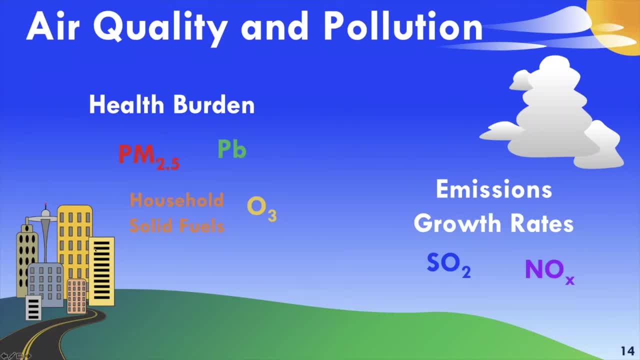 slide on air atmospheric chemistry, But the chemistry isn't the most important thing here. It's really what the issue that we check actually is, And what we do is we check the health burden. The units are disability adjusted life year rates, which is just a measure of morbidity and mortality from exposure to particulate matter. 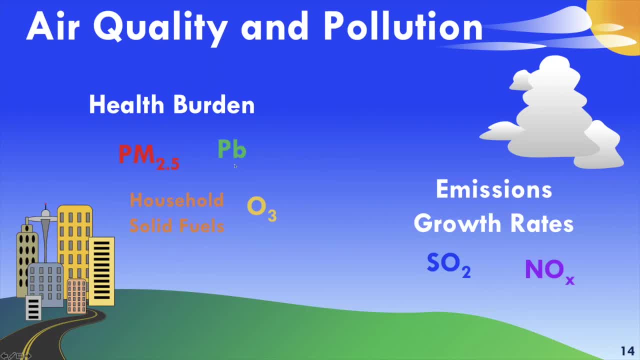 household solid fuel combustion, lead exposure and ozone. So in simpler terms, we just track premature death from these pollutants And then we also compute the emissions growth rates in other atmospheric pollutants like sulfur dioxide and nitrogen oxides. So countries that are emitting more and more of these pollutants receive a lower score. 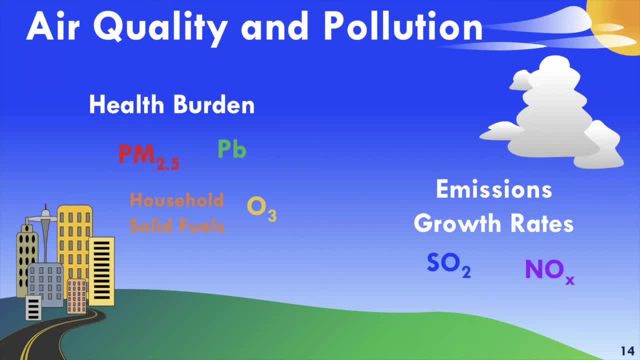 And you might also imagine that there's a lot of overlap between the kind of marine sciences implications and the atmospheric sciences implications of these trends. For example, I'm sure I don't need to explain ocean acidification, But by tracking carbon dioxide emissions as well as some precursors of acid rain emissions, we've now got a lot of 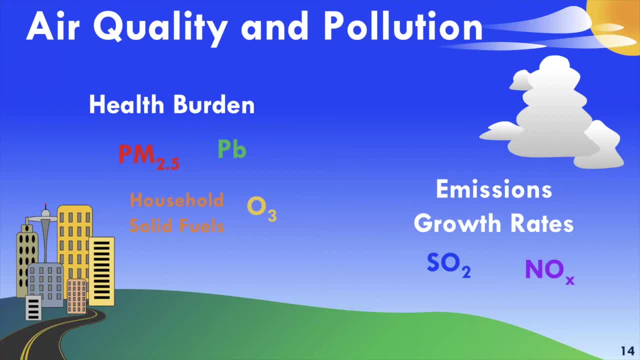 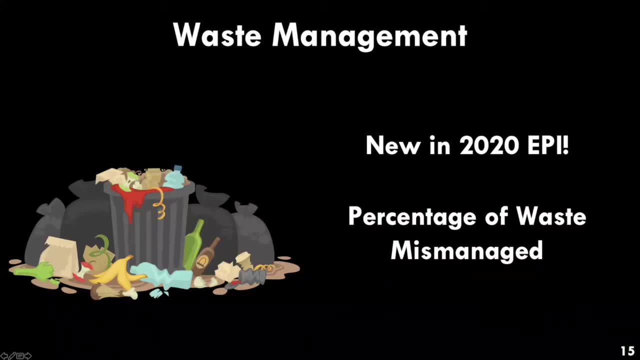 can, by extension, check countries' contributions to ocean acidification and things like that. So I'd also just like to specifically highlight a new indicator that was introduced in the 2020 Environmental Performance Index, which was waste management, So this has long been an issue on our radar. 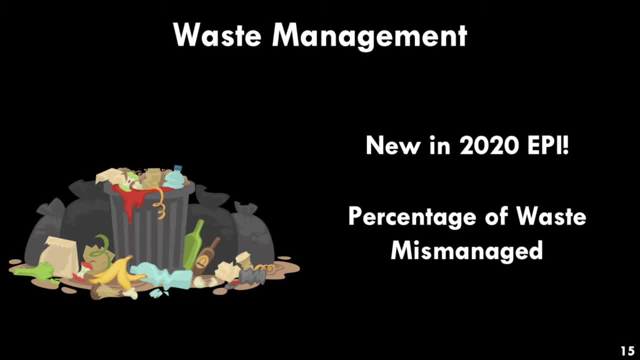 waste management has, But up until 2020,. we didn't feel that there was actually a good enough global data set. So in the last report, though the EPI team, led by Zach and others, they worked to incorporate the percentage of waste mismanaged, which is to say 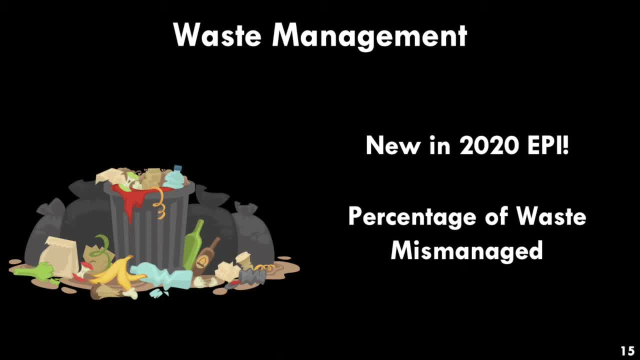 disposed of in unsanitary ways like open dumps and really substandardly designed landfills, as opposed to greener methods like recycling, composting and also sanitary landfills in each country. So we'll talk a little bit later on how I brought this up. 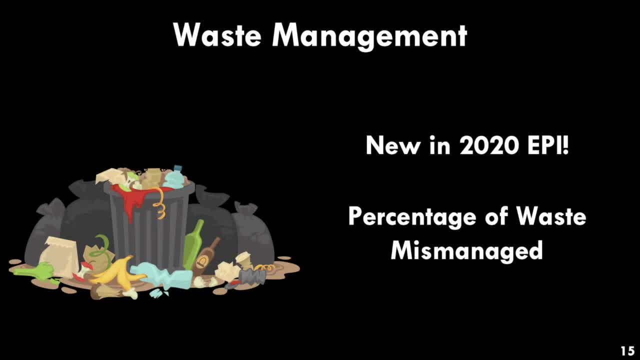 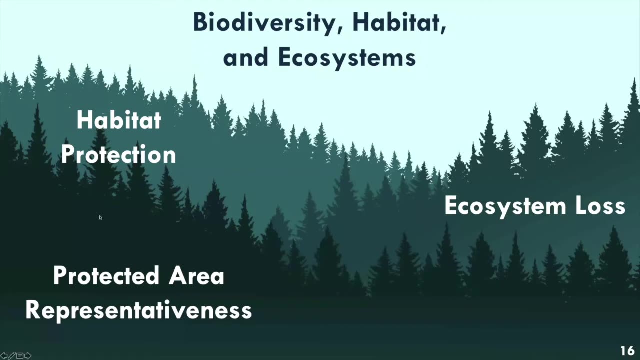 because we're also planning on extending the waste management issue category to also include things like ocean plastic pollution And the 2022 EPI, which might be interesting to some of you, And we also have several indicators relating to biodiversity and habitat conservation and ecosystem. 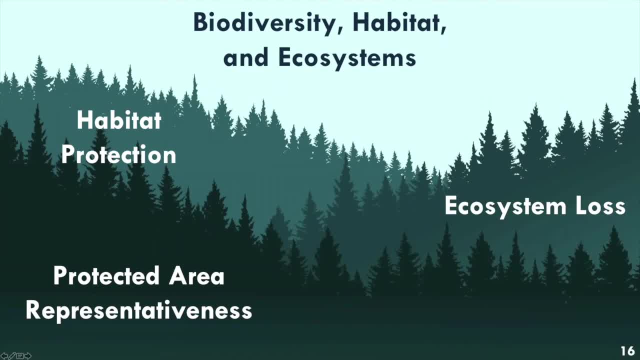 extent as well. So we not only check habitat protection itself but we also report how representative the conserved areas are to the habitat species that live within a country. So, for example, if a country is protecting a lot of grasslands but they don't have many species that live in grasslands, 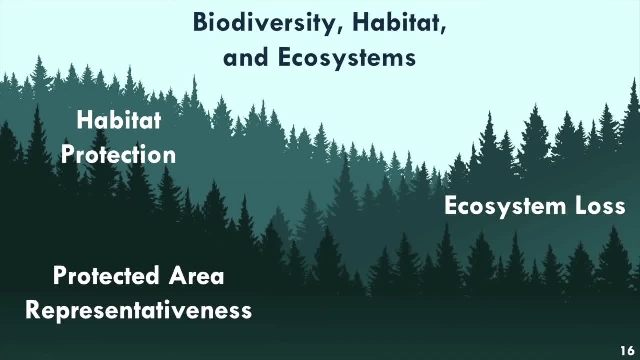 then they won't be rewarded as much as a country that's protecting the habitat that's directly needed by the species that live within its borders. And then also in our ecosystem services category, we check the loss of forests and wetlands and grasslands on a country level. 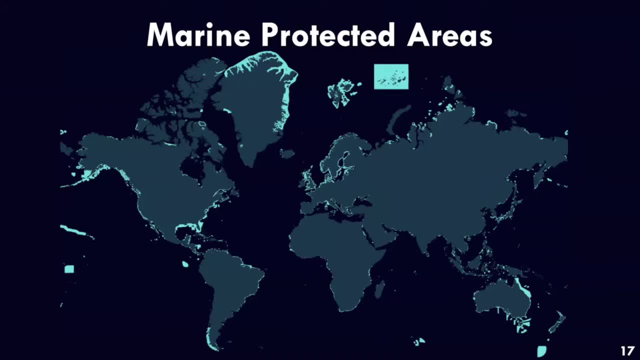 So I know that this is the Institute for Oceans and Fisheries, So I thought I'd specifically discuss some of our marine indicators, our marine indicators in particular. So the Marine Protected Areas indicator checks the percentage of a country's total exclusive economic zone, or EEZ. 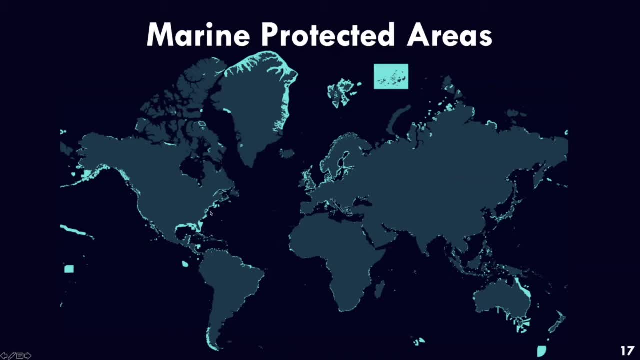 that lies within marine protected areas. So a top score on the Marine Protected Areas indicator means that a country protects at least 10% of its total exclusive economic zone area And that 10% comes from the IHEA target 11,, which is the country's. 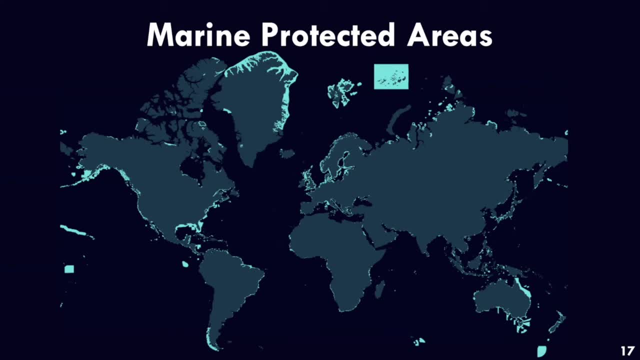 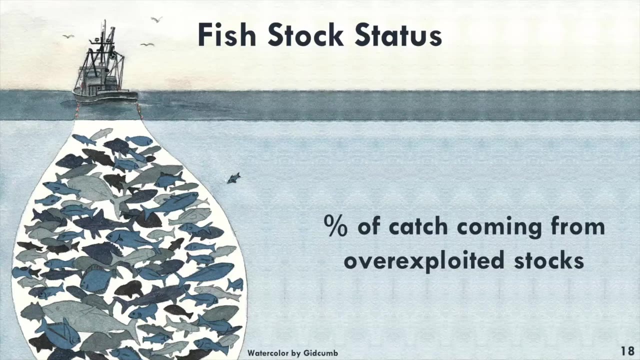 top 10% of the Convention on Biological Diversity, which says that, optimally, at least 10% of EEZs will be designated as marine protected areas. Oops, sorry about that, got to go back. So fish production and fish catch. 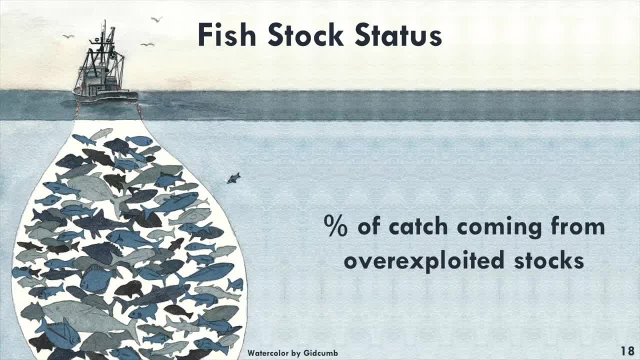 is increasing around the world, as I'm sure I don't need to tell you, And so we also report on several indicators that measure the sustainability of fisheries practices. So fish stock status in particular measures the percentage of a country's total catch. that 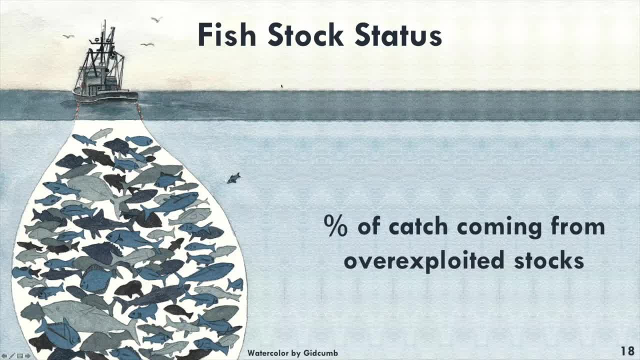 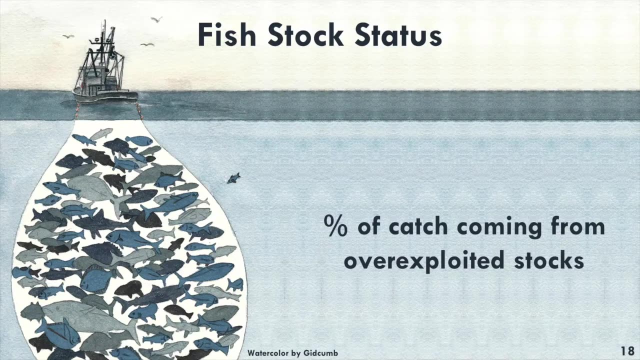 comes from either over-exploited or collapsed fish stocks, And a top score on the fish stock status means that 0% or none of a country's fish catch comes from fish stocks that are over-exploited or collapsed. We'll see later on that countries don't come close. 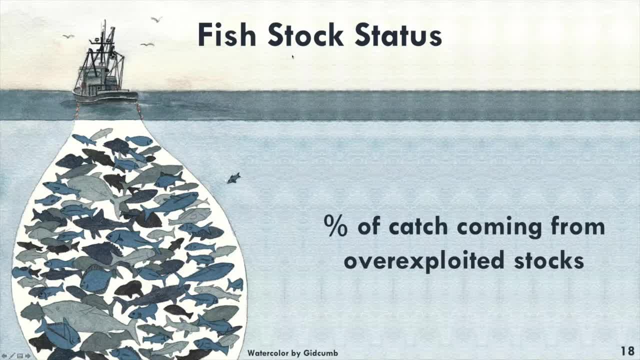 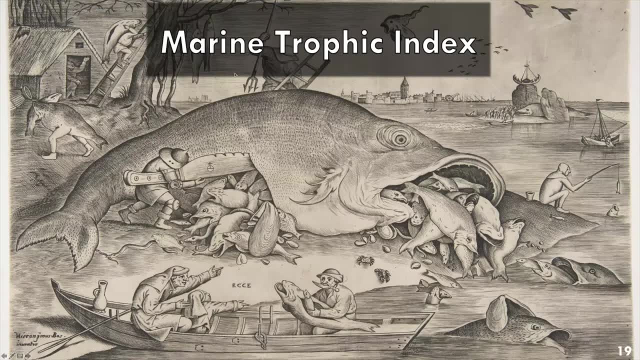 to achieving top scores. And the Marine Trophic Index, going further, measures the kinds of fish, So the big fish, that are being caught. I guess you could say So. this old woodcut by an old European, Peter van der Heijden, indicates what you might say. 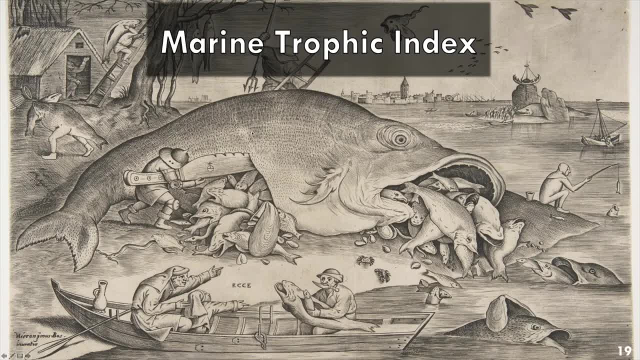 is a depiction of Marine Trophic Index. So the big fish here indicates a higher Trophic Index, whereas the littlest fish that is being eaten by everything else represents a lower Trophic Index. So countries that have a higher Marine Trophic Index score. 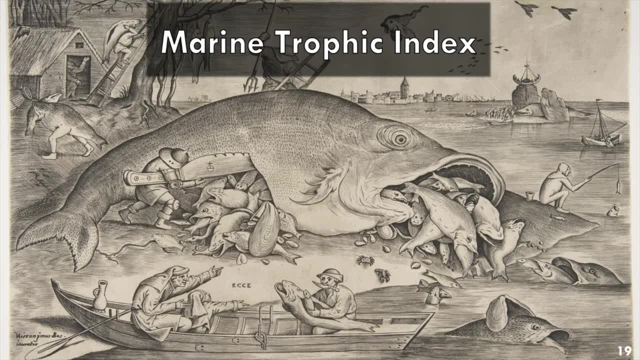 have fish catches consisting of species of higher Trophic levels, while lower scores of Marine Trophic Index indicate the species that are being brought in further down the food web. So if MTI Marine Trophic Index decreases over time, 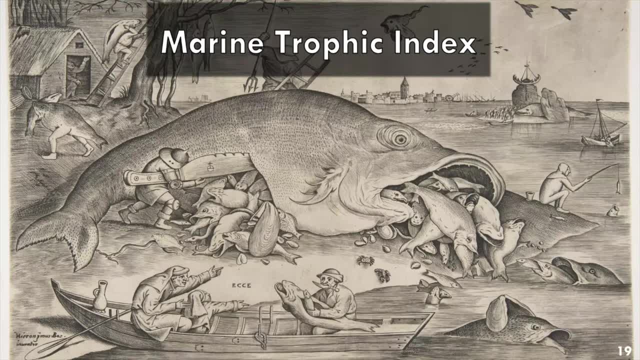 this may be due to the fact that countries are depleting stocks of higher-level fish and resorting to bringing in lower-level taxa, which is also known as fishing down the food web, And if countries are bringing in fish that have legs and feet on them, then they. 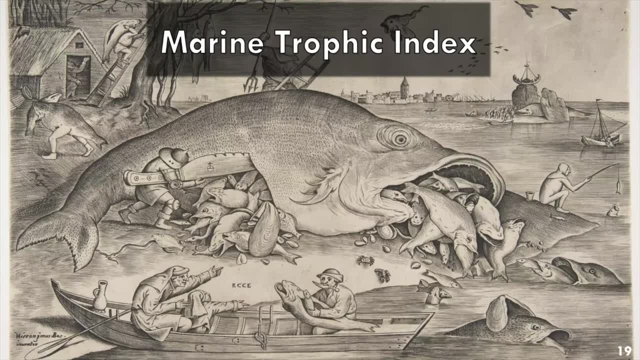 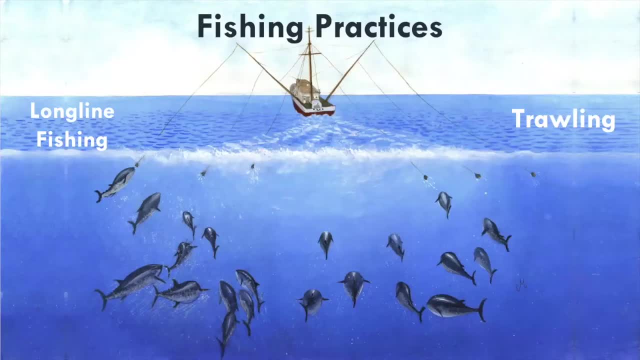 might be fishing in very polluted waters, but that's not something that we consider in the API. So we also recognize that different kinds of fishing practices have disparate impacts on ocean ecosystems. So some, like longline fishing that's illustrated here, are more discriminant in the kinds of fish. 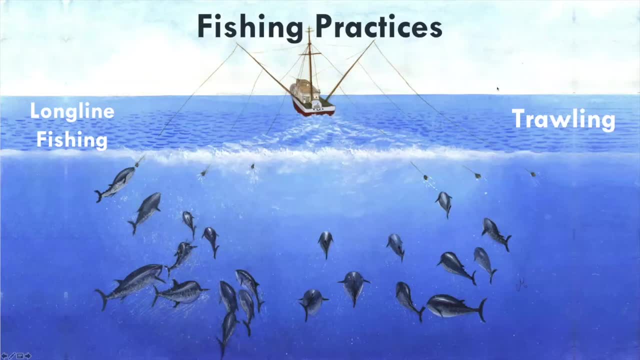 that are being caught, which is good. Trawling, on the other hand, just drags nets through the water or along the bottom floor, which indiscriminately catches fish, Resulting in a lot of wasted bycatch. It can also damage sensitive ecosystems. 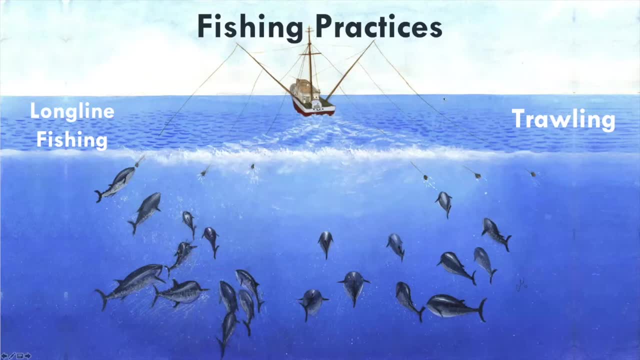 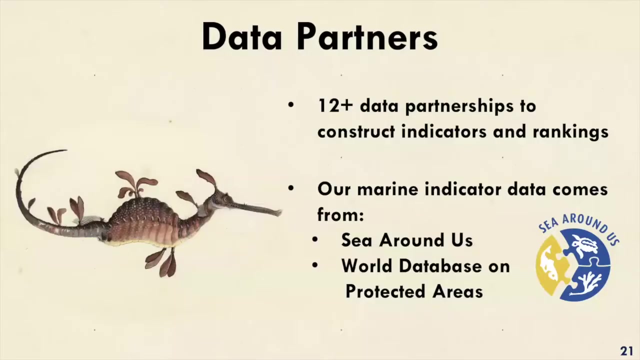 that the ocean floor that fish rely on for responding and reproduction. So the API has an indicator- fish caught by trawling- which measures the proportion of fish caught using trawling methods. So this is the slide that Ding has probably been waiting for. 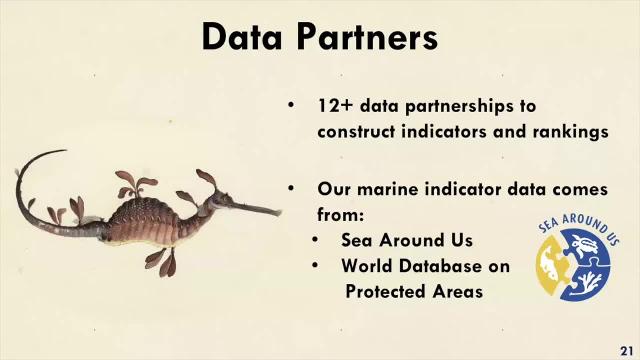 But we're not really in the business of collecting data ourselves. Rather, we actually rely on databases and collaborations with many different data partners. So the API currently has over 10 or even over 12 different data partners that we use to get relevant data to construct. 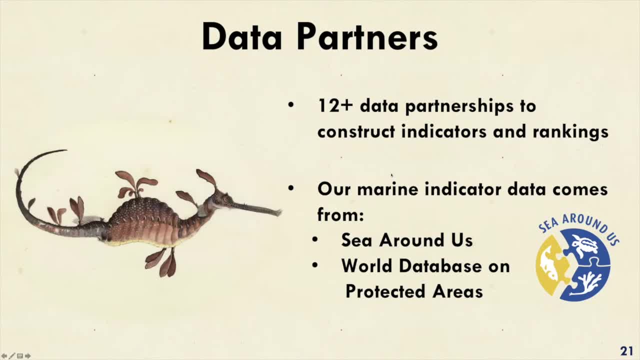 our indicators and our rankings. So all of our fisheries indicator data comes from the Sea Around Us initiative right there at the University of British Columbia. So we're really grateful to have this collaboration with Ding and Daniel Pauling and others at the Sea Around Us. 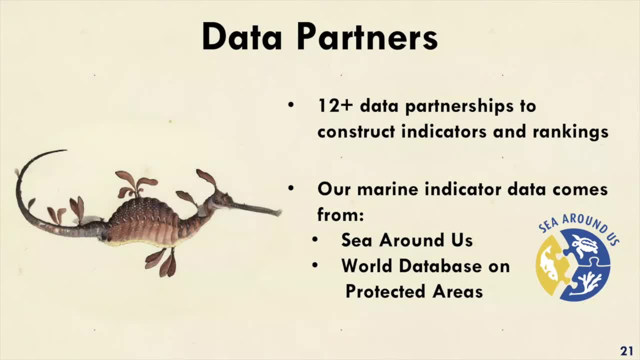 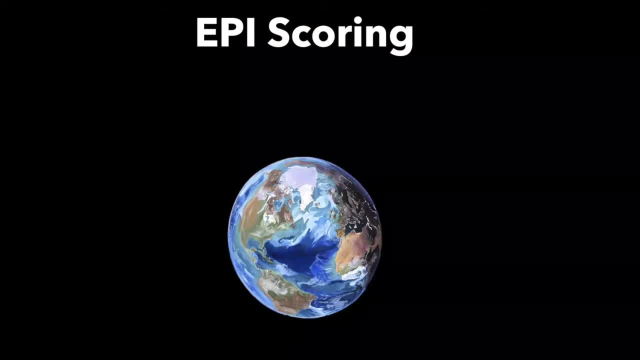 for the great work that they're doing and also for providing us, And we're also really grateful to have the critical data for our analyses. OK, so that's a very quick and fairly broad overview of the kinds of environmental issues that the API considers. 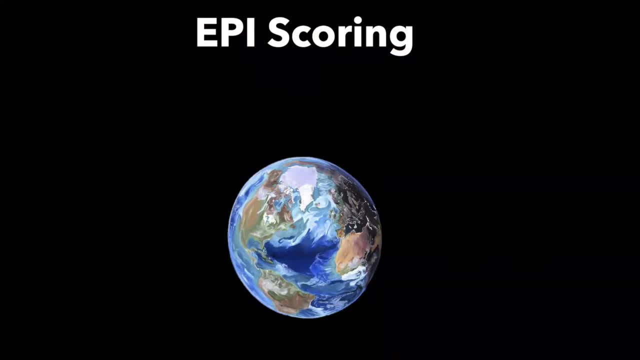 But now we'll come to the next question which might be on your mind, which is: how do we go from these global data sets to our rankings, where we compare countries' environmental scores against each other? So overall, we have three main guiding. 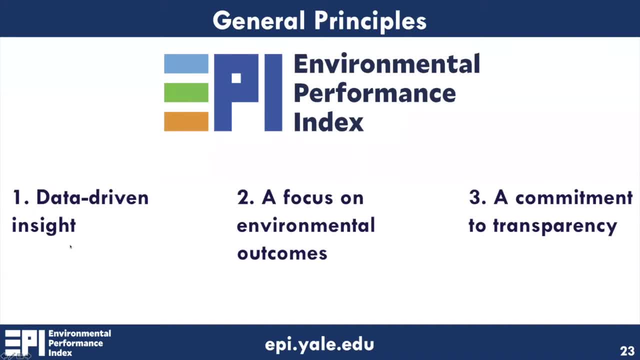 points in the API's methodology. So, first, we don't rely on anecdotes to inform our rankings and conclusions, but rather we rely on data-driven analyses. So data and facts are really important to us. And second, we focus on environmental outcomes rather than policy inputs. 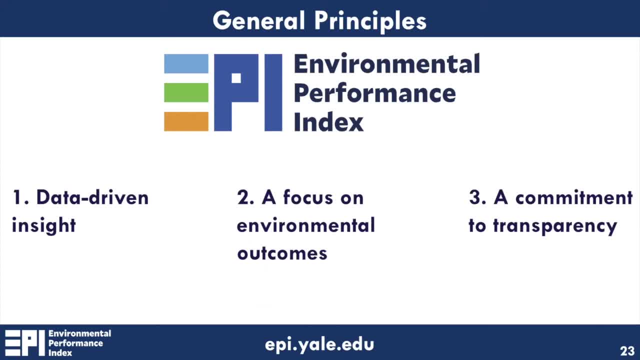 So that is to say, we don't reward countries for simply having environmental policies in place or codified into law. Rather, these policies need to be actually effective And we focus on improving their environmental performance in a category in order for a country to earn a high API score in that category. 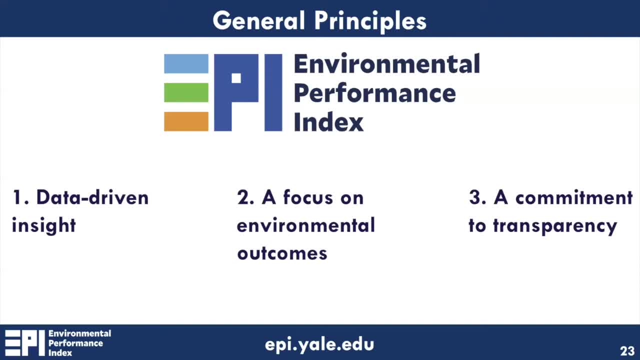 So just having policies is good enough. The policies need to be effective. And, finally, we also uphold a commitment to transparency, So we publish all of our data and our methodologies and are always open to discussing our work with interested parties, like you. So thank you. 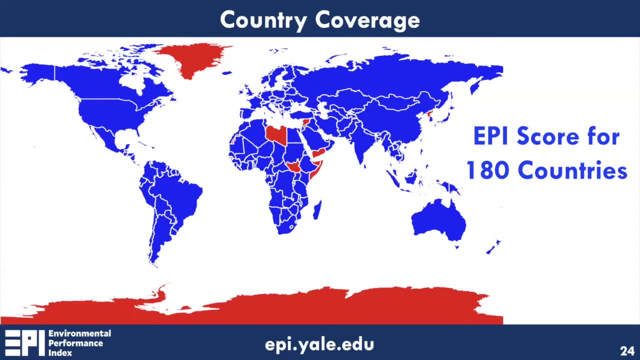 Taking into account Data coverage and also quality, we're able to compute an overall API score for 180 countries around the world in the 2020 Environmental Performance Index. Sometimes we have data for maybe a few indicators for some of the missing countries. 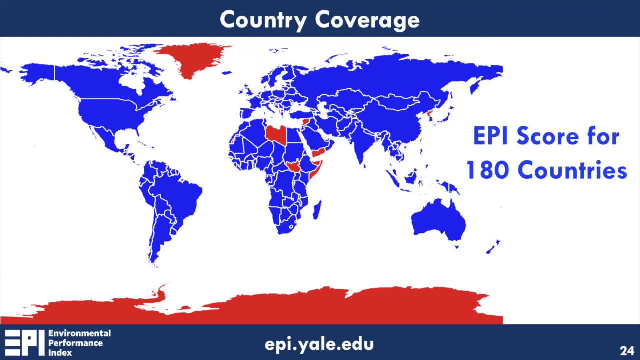 but not enough data to calculate a reliable overall Environmental Performance Index score. Just for example, we don't compute an API score for North Korea. Although we have satellite data on air quality data and forest loss data, The North Koreans don't report other necessary data. 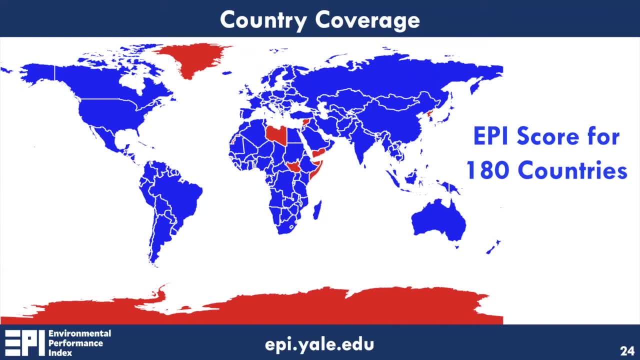 to international organizations like the United Nations Environment Program, for example, We don't have enough data to compute a score for that country. However, we're always looking for more comprehensive and robust datasets, with the goal that one day we'll hopefully be able to compute a score. 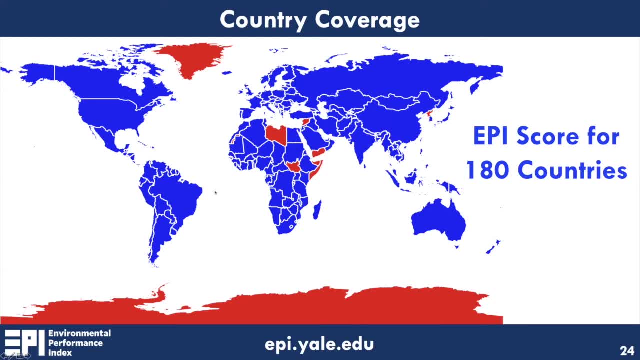 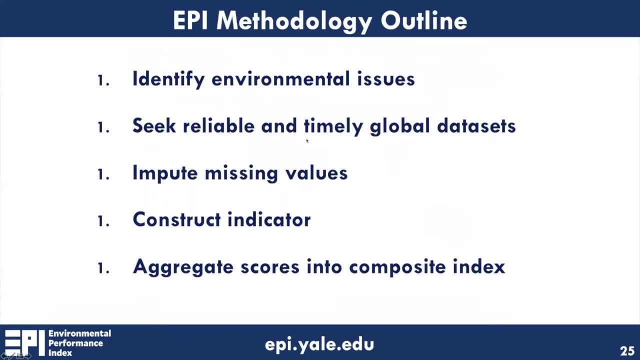 for over 200 countries. Especially, we are working to include data sets that report on kind of small island nations that are traditionally overlooked. We don't think that's fair. We want to bring them into our analyses as well. So here's just a very quick and brief overview of our methodology that we follow for each iteration. 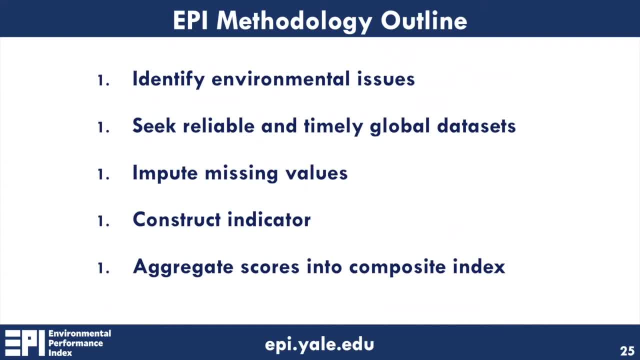 of the EPI, so every other year. So first we really take a step back and ponder what important environmental issues are out there that we ought to try and track. Then we try and seek recent and robust global data sets that address all of these issues that we're considering And for some issues, 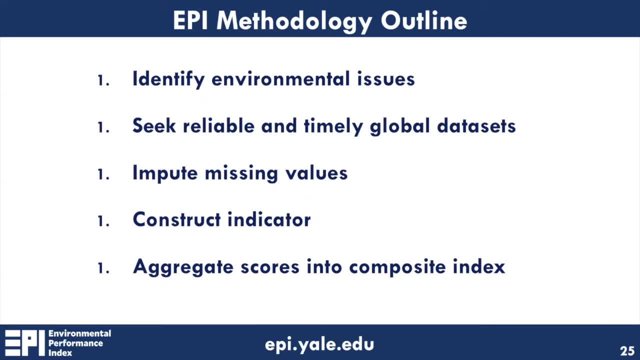 the idea has to die there just because there aren't good enough global data sets on the issues. But the ones that make it through our team can sometimes work to fill gaps, where possible through predictive models and interpolation. But then we move on to compute. sorry, 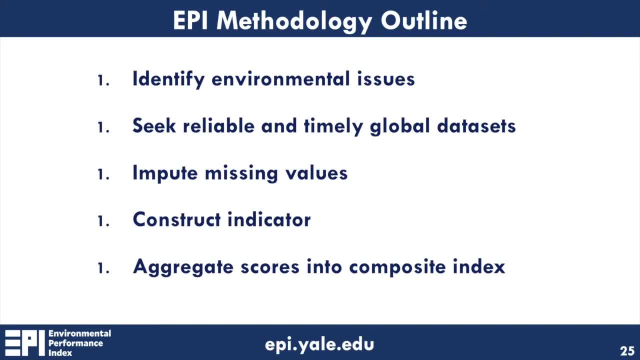 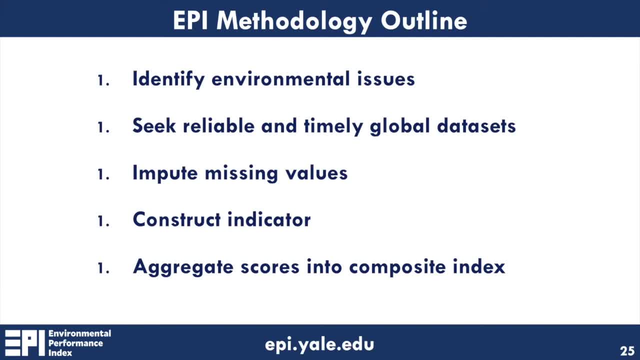 So the indicators give each country a score between 0 and 100, 100 being the best score. And then, finally, we take all of the individual indicator scores, so all 32 of them, and aggregate them into a single final API score: that. 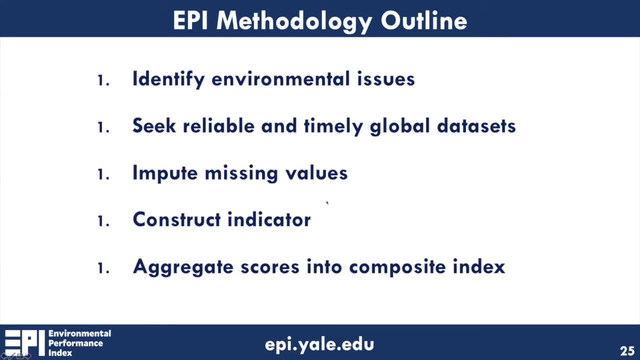 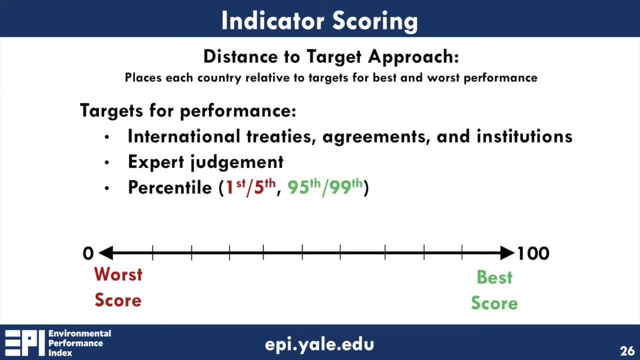 succinctly summarizes each country's environmental performance. So, as the last slide may have insinuated, one of the really crucial steps in indicator construction, it is determining what the best and worst scores should be. So the API uses something called a distance-to-target approach. 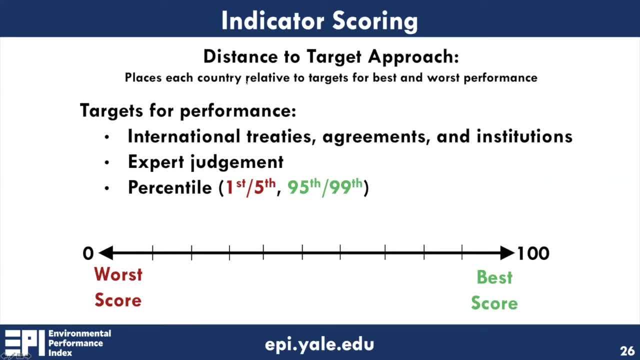 where a country's score is determined by how it performs relative to certain targets. So the targets are ideally determined by things like international treaties and consensus, maybe agreements or accords or intergovernmental institutions, For example the IHA target 11.. 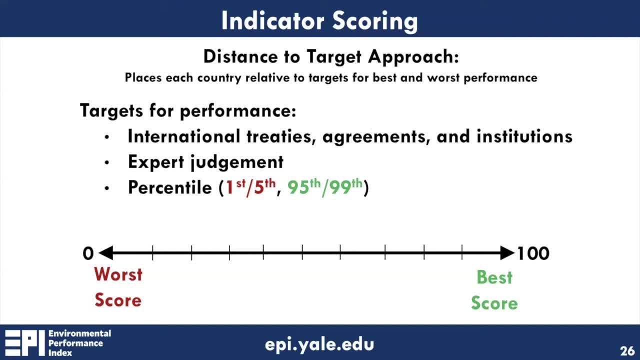 of the Convention on Biological Diversity stipulates that a country should designate at least 10% of its exclusive economic zone as marine protected areas. So if a country has 10% of its EEZ as marine protected areas, it would receive a top score of 100%. 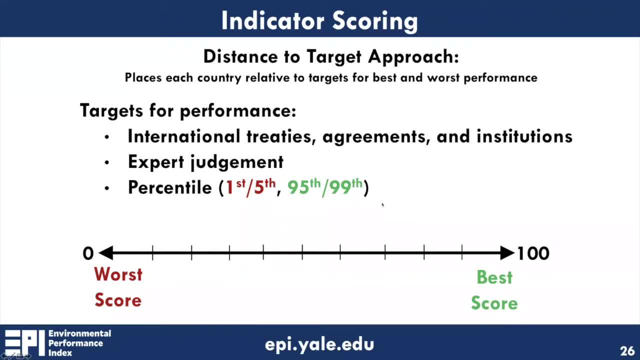 because it's met that international consensus. In the absence of targets that are set by these international agreements and consensus, though, we turn to targets set by expert judgment, which is sometimes reported in the literature. Or, lastly, we start by relative performance. 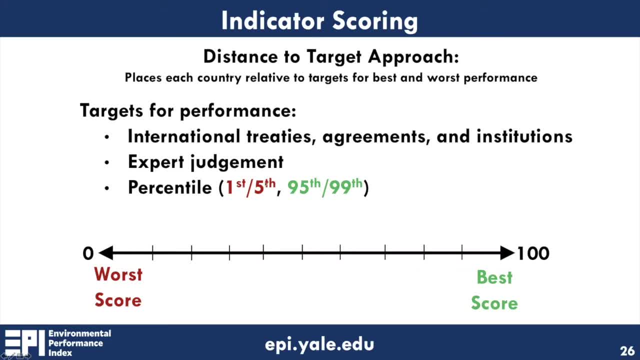 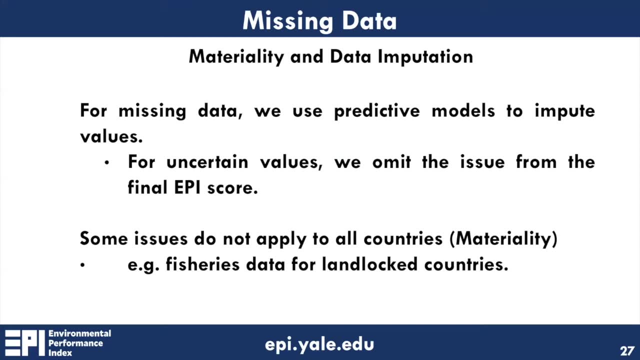 which is to use percentiles, so the first or fifth percentile for worst performance or 95th or 99th percentile for best performance. So, despite our best efforts to look for comprehensive data sets, sometimes the data is unfortunately missing. So where possible, we use regressions. 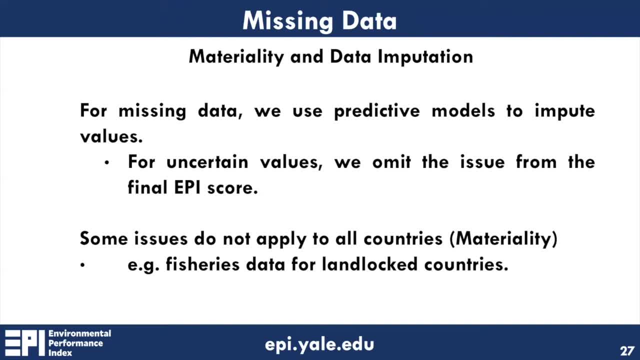 and predictive models to try and interpolate or impute a country's score, But if we feel that we're unable to do that accurately or rigorously, we'll instead leave that indicator out of a country's CPI calculation and redistribute the weight that's normally given to that missing. 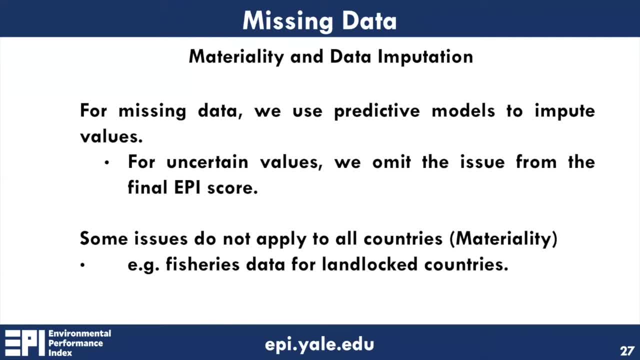 indicator to other issues And we'll get to weighting in a few slides. Sorry, it might be a little bit confusing, but it will become clear in a figure in the next couple of slides. I should also just mention that some issues don't. 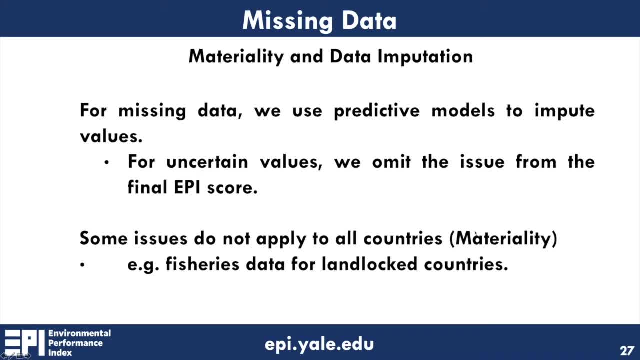 apply to all countries. So we call this a materiality A filter. It's wonderful talking to a group like you, because fisheries is a really great example of a materiality filter. So fishing indicators don't really apply to landlocked countries, at least not the fishing. 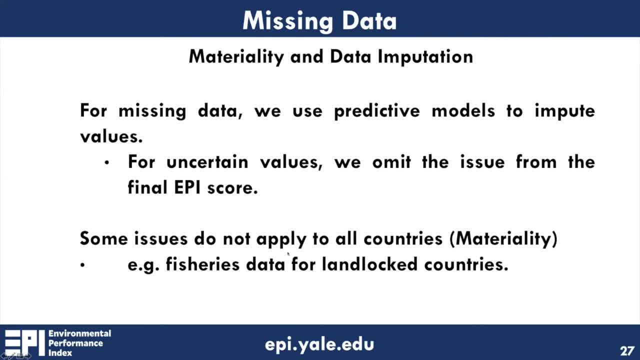 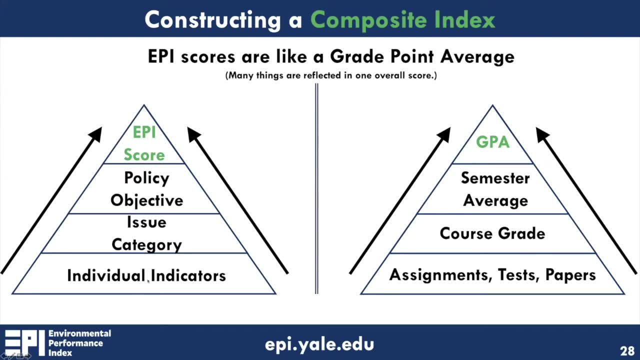 indicators that we use. So in this instance we also redistribute the fishery indicators contribution to the final EPI score to other indicators that do apply to these countries. So once we have scores for each individual indicator, we then compile the scores into issue categories. 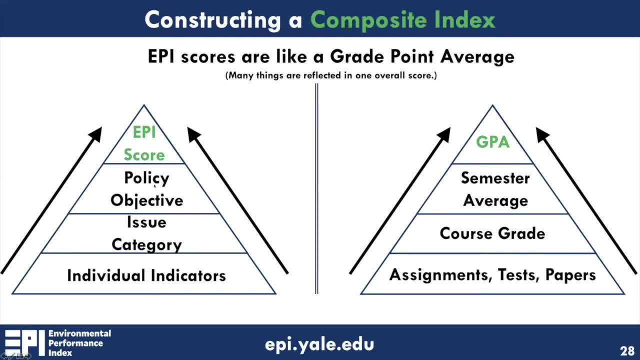 and then the policy objectives, which were environmental health and ecosystem vitality, you might remember, and then finally into an overall environmental performance index score. So this process of taking many individual scores on specific environmental issues and then calculating a single overall EPI score, we like. 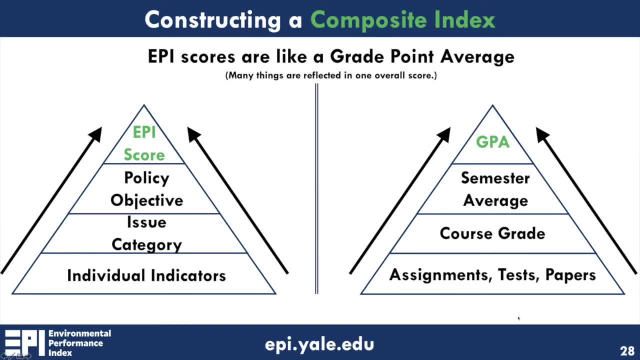 to think that it's analogous to a student's grade point average. So a student gets many scores And then they get a score. So a student gets many individual grades on assignments and tests and essays, et cetera over a semester, which then get compiled into a course grade. 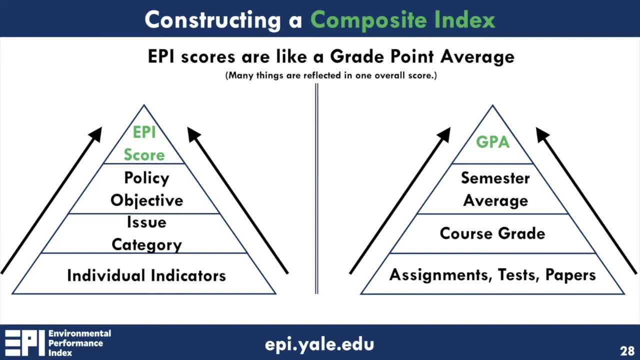 But then a student takes probably several classes each semester And each class grade is compiled into an overall semester average And then finally a multi-year grade point average. So one thing I just want to emphasize here is that we don't only report a country's final overall EPI. 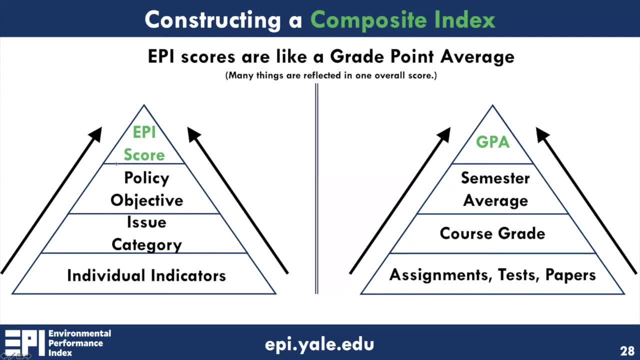 score. We also report its performance and its rankings at each level below that. So its policy objective scores, issue category scores and individual indicator scores, which we hope allows countries to really delve into the details to see how relative to their peers on specific issues. 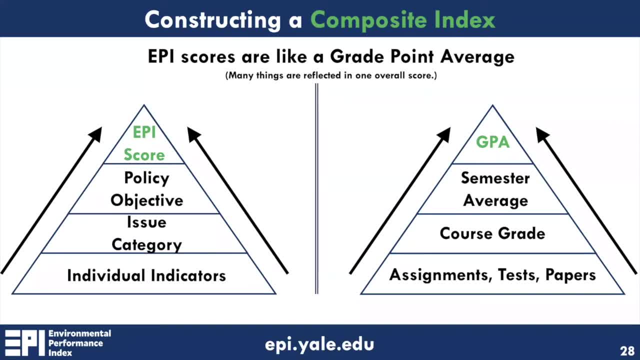 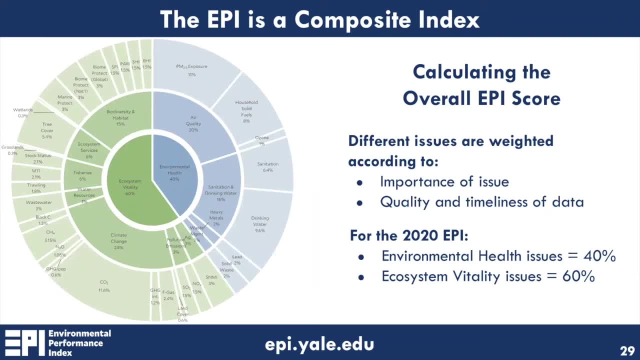 that they care about as well as more generally. So, to aggregate these issues into a final score, I'm going to assign each issue a specific weight or a percentage of the final score which this wheel demonstrates for the 2020 Environmental Performance Index. 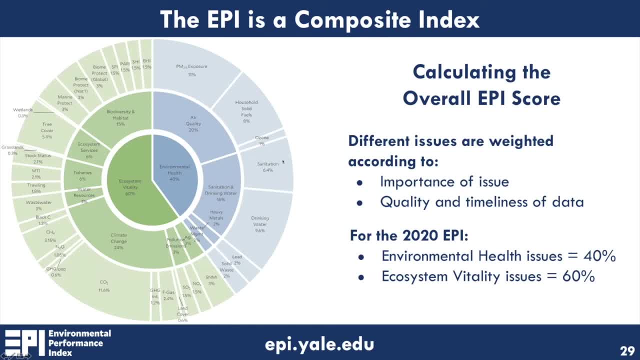 So on the outside of the ring here, we can see each of the 32 different individual environmental issues that we check, grouped into their 11 broader issue categories, which are then grouped into their policy objectives, And one thing that you might be questioning is: why are some? 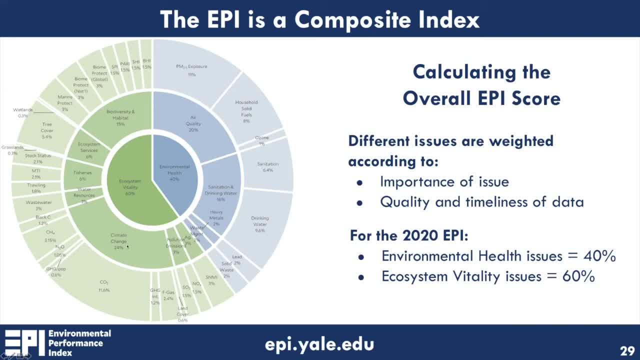 issues given grade? Why are some issues given a greater weight than others And how do we really determine this weighting scheme? So, just for example, climate change. that might be hard to see on the slide, but climate change is given 24% weight of the total overall EPI. 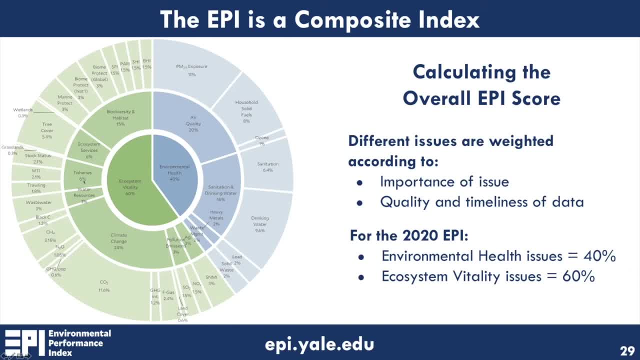 score, whereas fisheries, I'm sad to report, is only given 6%. But how do we actually come up with these numbers? What we do? well, I can say that the weighting is dependent on a couple of different things. More important issues as determined by expert judgment. 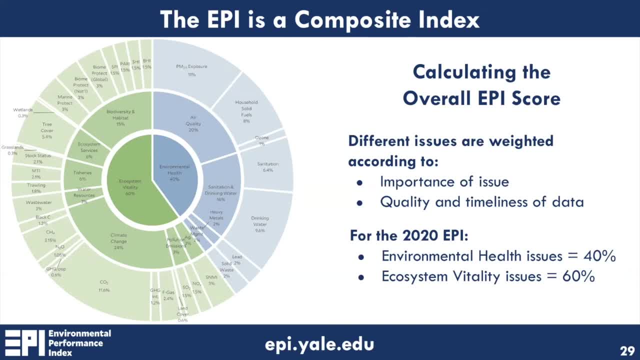 and kind of expert consensus, are given greater weights. So periodically we convene panels of experts, give them 100 points and say: OK, you have 100 points. 32 different indicators assign different amounts of weight to each issue. 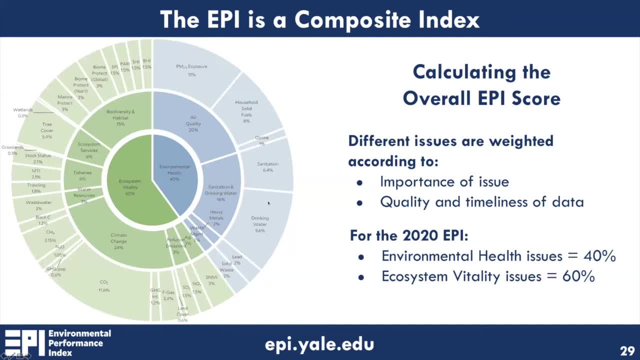 And then we can go and try and resolve differences if there's great discrepancies between that. We also take into account the quality and the time beingness of the data. So, for example, if we have an important indicator, an important issue, but the data is getting quite old, 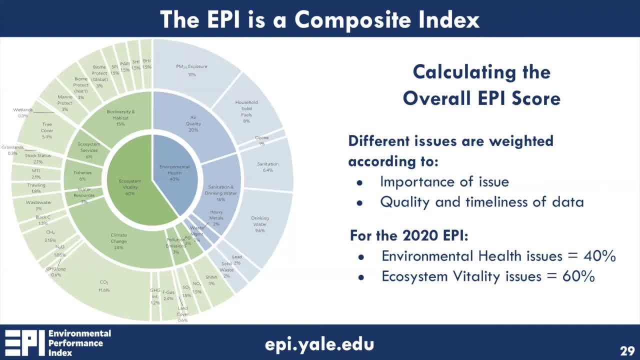 maybe six, eight years back into the past, We'll down weight- the importance of that- in the overall weighting scheme, because countries and their policymakers are particularly interested in the most recent data to know how they've been performing recently, perhaps since new environmental policies have been enacted. 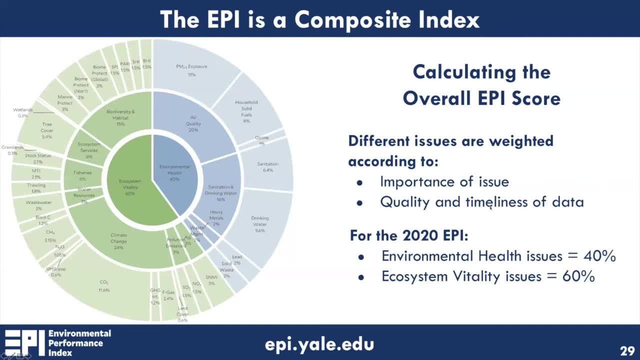 Right. So both the importance of the issue quality and the timeliness of the data factor into the overall weighting scheme. We have done some sensitivity analyses which we encourage you to explore in our technical appendix and in our audit. You can find all of that on our website at epiyaleedu. 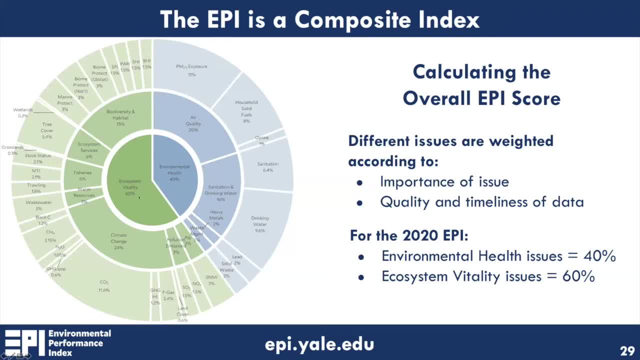 where we vary the weight of each of the different indicators And we find that overall, the country's rankings are fairly insensitive to the amount of weight given to each issue, because countries tend to do well or worse on all issues collectively. But it's an important question to ask. 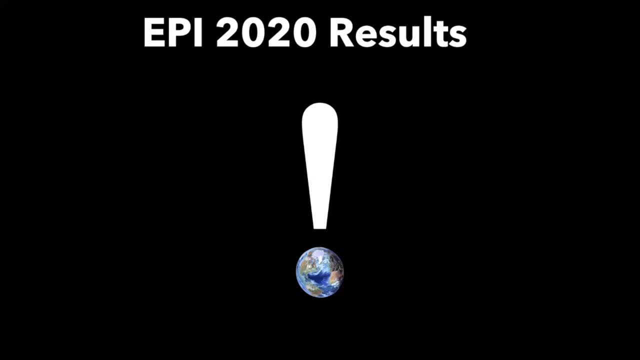 OK, so now that we have some understanding of how we compute environmental performance index scores, we can turn to what I think, hopefully, will be the exciting part of the seminar, which will be showing and sharing some of our results from the 2020 Environmental Performance Index analyses. 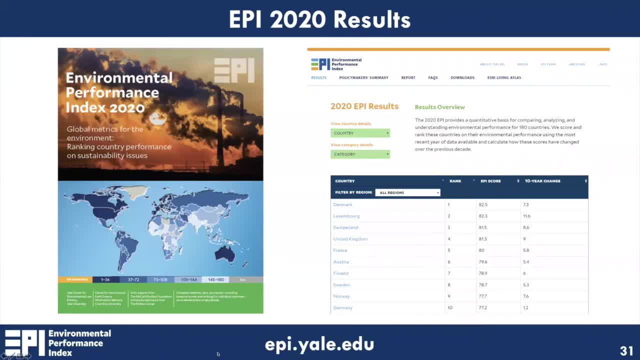 So we encourage you to explore the results in more detail on our website, epiyaleedu, And if you go there, you can find the 2020 report, the overall rankings and also rankings for each of the 32 different environmental issues. 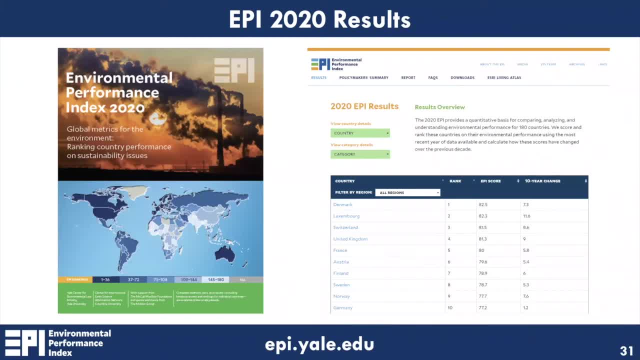 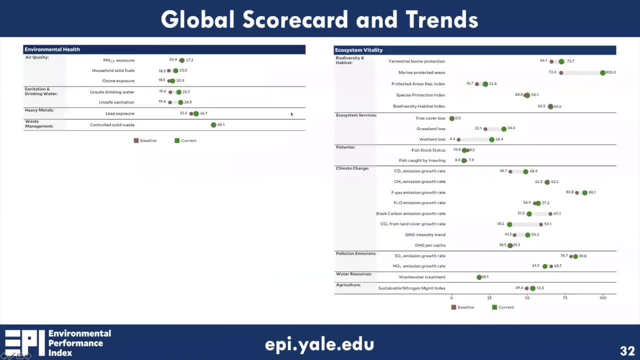 that we talked about earlier. So if you're interested in how a specific country does in a specific issue, we try to make it easy to explore that data in our country's scorecards. So I'm just sharing some of the broad results with you. 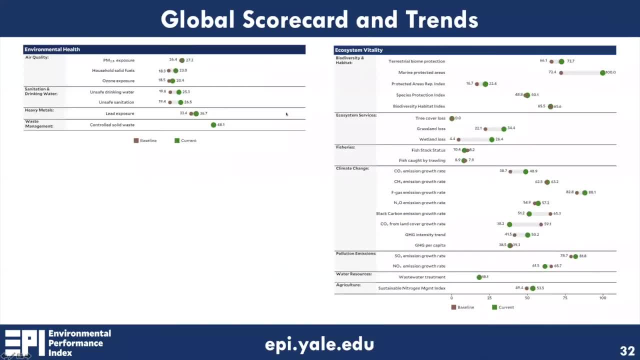 We can first take a look at our global scorecards and trends. So what we show here is the current EPI score for the globe in green, as well as what the EPI score would have been approximately 10 years ago if we applied the same methodology and data. 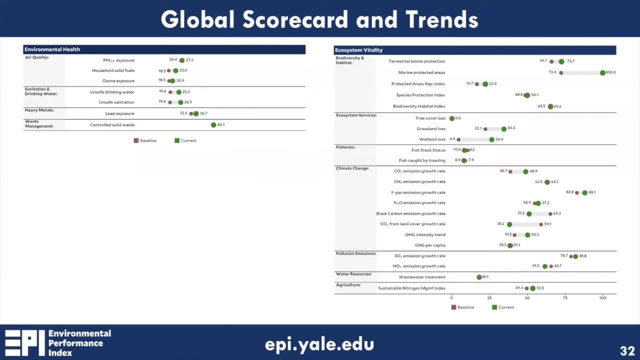 sources to decade-old data, the same weighting to about decade-old data. So there's both good and bad news. you can see The world as a whole has been making fairly good progress, especially in the last few years, And we've seen a lot of progress towards protecting. 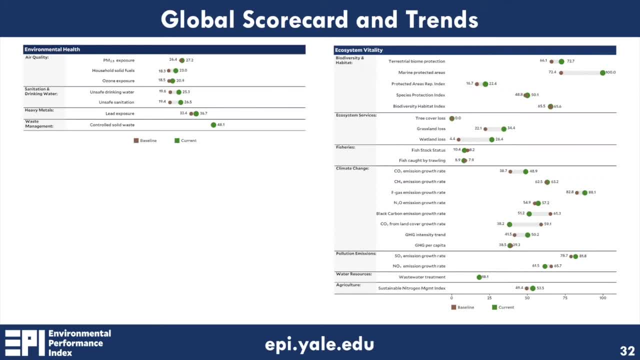 marine habitat, which is good, Although, as we'll see later, there's certainly some individual countries that still are falling behind in this area, And there's virtually no change, maybe even a slight decrease, in global fish stock status and fish caught by trawling. 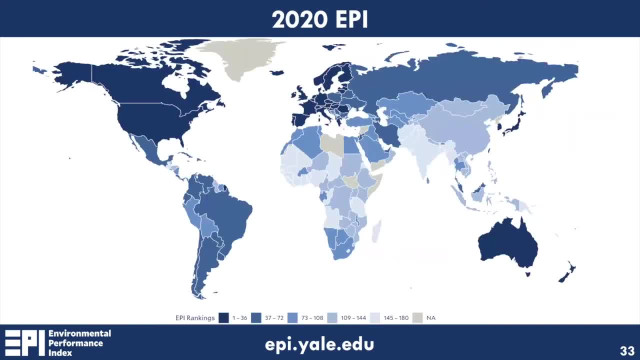 And this indicates that we still have a lot of work to do to improve fisheries practices worldwide. The graph just shows overall EPI ranking by country, with darker blues indicating better performance, And we can see that the more developed countries, specifically North America and Western Europe, do well. 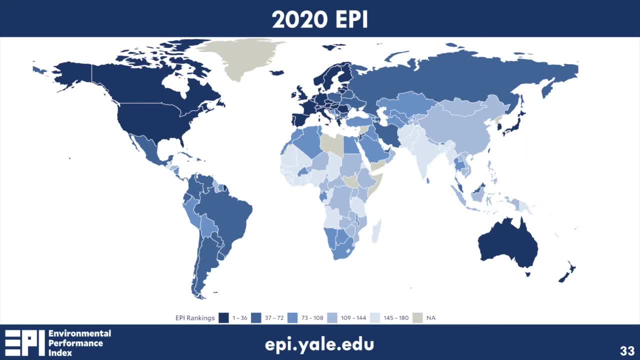 whereas developing and underdeveloped countries that have fewer financial and political capital to dedicate towards environmental protection receive lower scores. But this isn't really the most important conclusion of the EPI. We hope that, if you only take one thing away from the seminar, 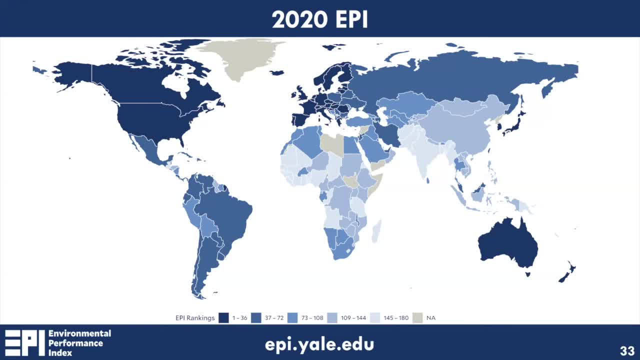 it's this. One of the most important applications of the EPI is that it can be used to compare scores not across all countries, but rather between peers or peer groups. So these are the overall leaders, And we can see that Denmark was number one. 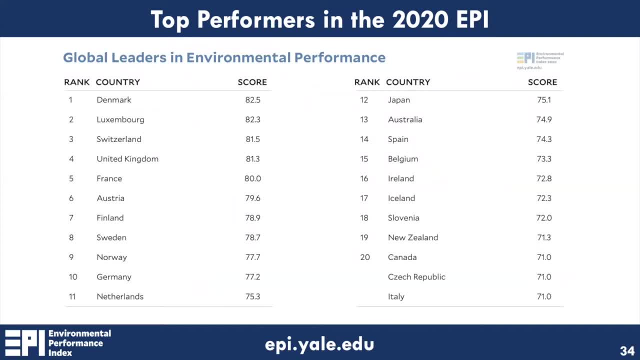 Canada was tied for 20th and the United States was 24th. So even though 20th place out of 180 is good and 24 out of 180 is good, we're still falling behind our peers. So we're trying to make it very easy to compare countries. 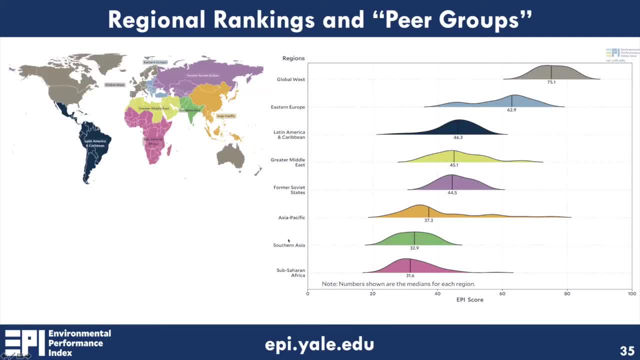 to their peers, And we also recognize that it's not necessarily fair or equitable to compare developing countries to developed countries. The disparity in resources and capital, et cetera, will of course result in varying degrees of environmental performance. It is interesting, though, to compare countries. 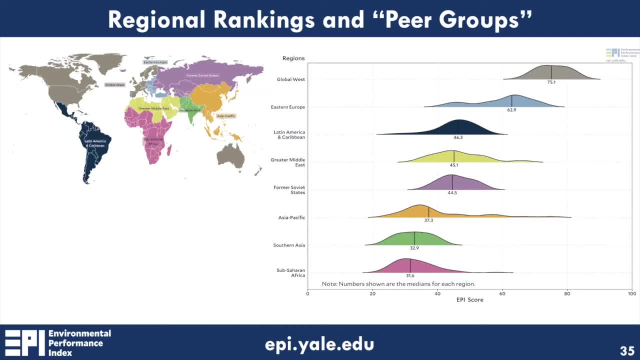 to their peers both by region and also by peer group. you can see, So some of our first-pass peer groups simply separate out countries by economy or by region, or by region, Or by wealth, or by geography, or also by common history or culture. 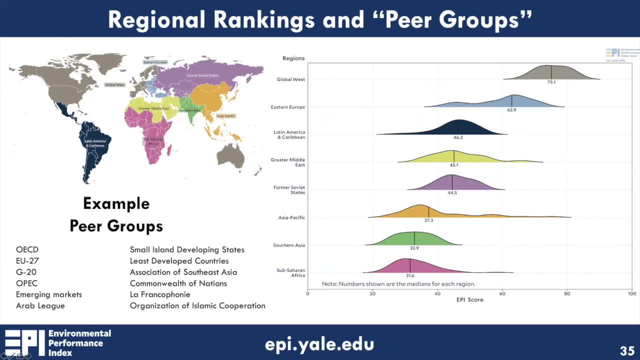 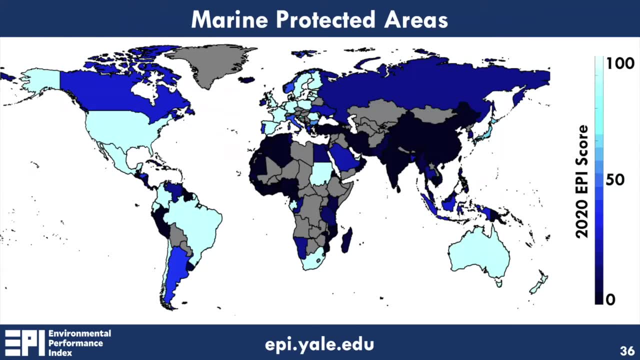 So we really encourage you, if you're interested, to go and explore these results and comparisons in greater detail. So in the last what? maybe five minutes or so, I'd just like to briefly share some results pertaining specifically to our marine indicators. 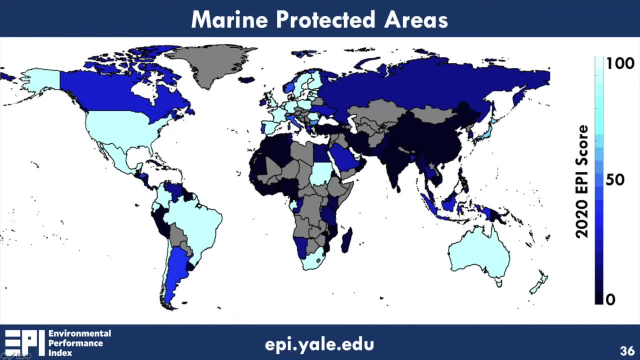 So this map shows the distribution of EPI scores on our marine protected area indicator. So scores of a zero: Zero is the worst score and 100 is the best score you can see. So, importantly, the marine indicators don't apply to all countries, particularly landlocked. 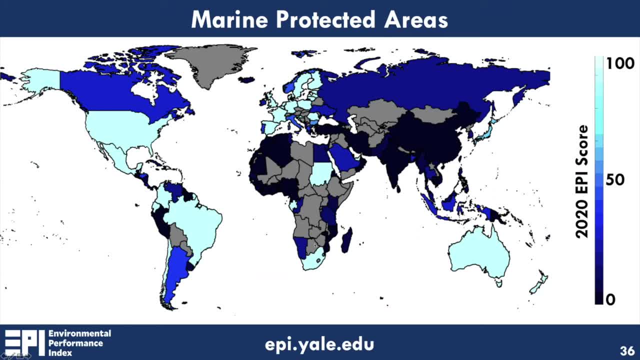 countries In other times. we just don't have enough reliable data to compute the score for each and every coastal country. Generally, though, you can see that the results are, I guess you could say, kind of bifurcated right. 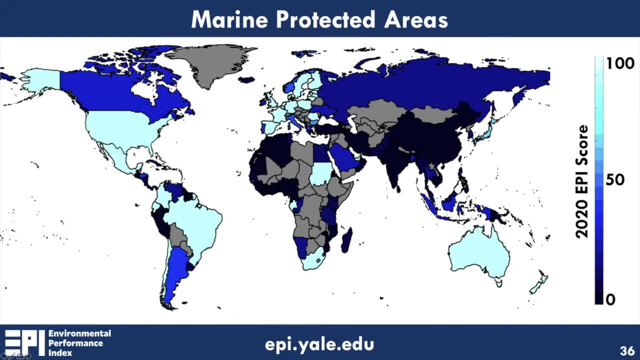 Many countries- the ones highlighted in light blue, like Brazil and Mexico, and the United States- have met or or exceeded their marine protected area goal of 10% of their exclusive economic zones. Many other countries, however, particularly in Southeast Asia. 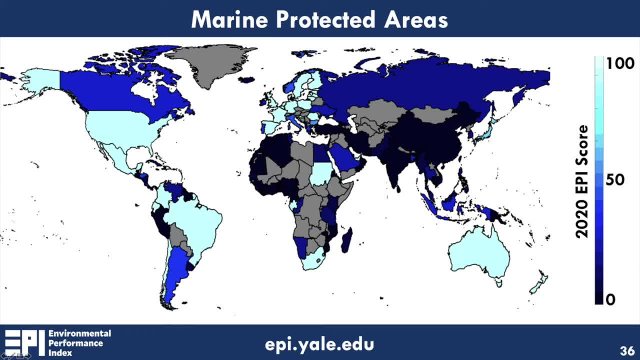 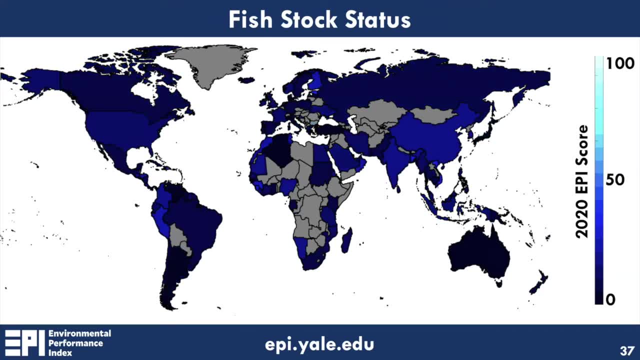 and Western Africa are falling well below the goal. So, while some countries are actually meeting their marine protected area goals, I think it's pretty much safe to say that no country is close to the optimal performance in terms of fish stock status which, as you recall, measures the proportion of a country's total catch coming from landlocked areas. So that's the goal. So I think it's pretty much safe to say that no country is close to the optimal performance in terms of fish stock status, which, as you recall, measures the proportion of a country's total catch coming from landlocked areas. 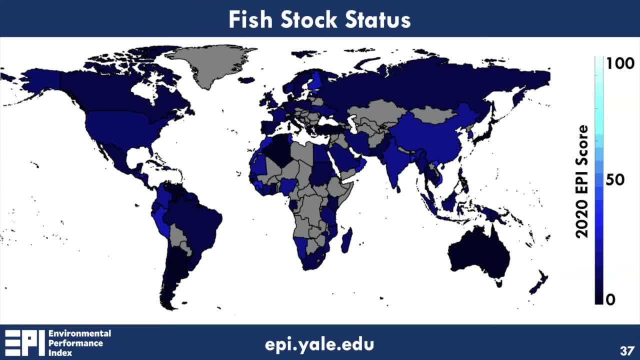 fish stock status which, as you recall, measures the proportion of a country's total catch coming from landlocked areas, over-exploited or collapsed fishing stocks. And, in fact, the best performing country, according to our data from the sea around us, is Estonia. 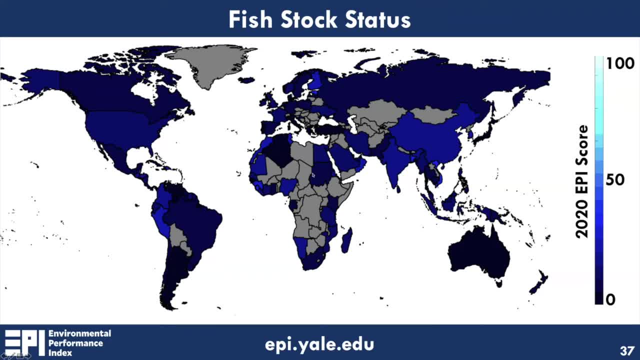 which really only receives a score of 36 out of 100.. So you know, it's safe to say every country needs to enact better fishing practices to reduce ecological pressures on over-exploited fish stocks. Moving on to another marine indicator: fish caught by trawling. 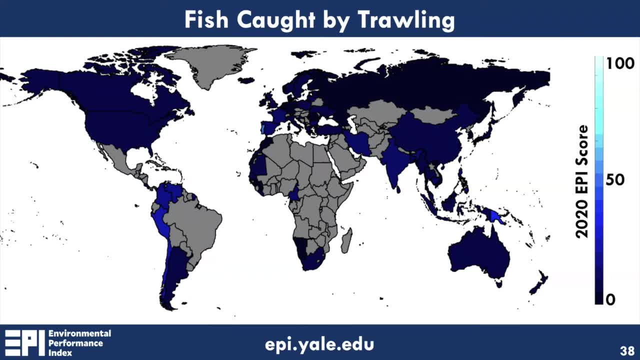 We can see a similarly- you might call it a dismal- picture. right, A score of 100 percent or 100 indicates that no fish are caught by bottom or pelagic trawling, whereas a score of zero is worst performance, measured by the 99th percentile proportion of fish caught by bottom or pelagic trawling. 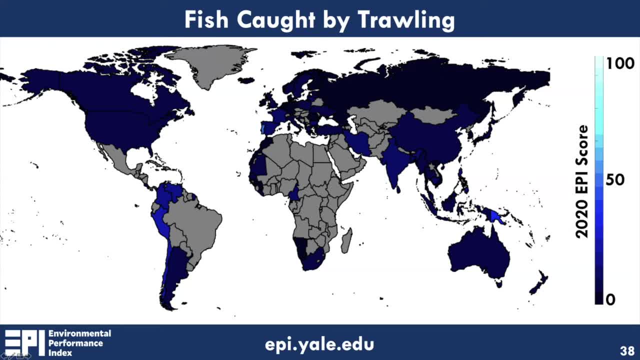 So again we see relatively uniformly poor performance in most countries. There are some exceptions, though It doesn't really come through on this map, But many small island nations like the Maldives or Singapore receive a top score of 100,. 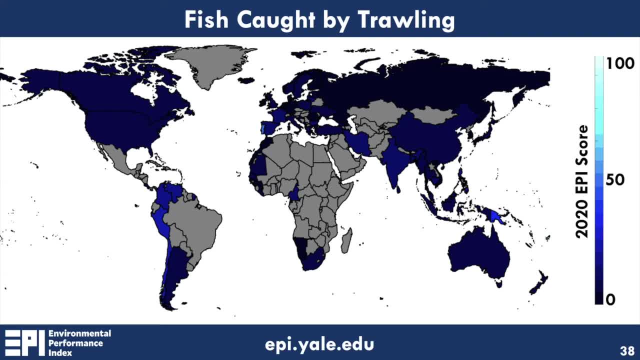 meaning that they catch no fish through trawling. So our results indicate that most major countries, countries that aren't small island nations, have much room for growth, to put an optimistic spin on it. And then, finally, due to some data constraints, 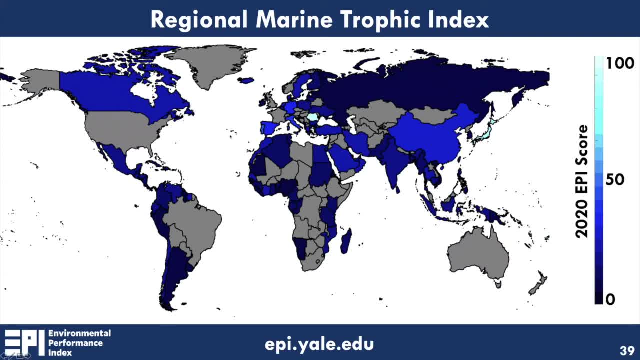 we weren't able to universally calculate Marine Trophic Index scores for all countries, But the indicator here represents Marine Trophic Index, 100 being no decline in marine tropic index over recent years and a score of zero indicating the sharpest decline. 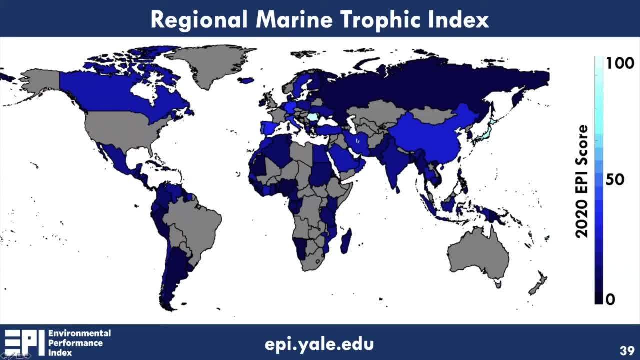 in marine tropic index And there are some middle performing countries here. but again, there's much room for improved fishing policies that regulate by catch, et cetera, to ensure that taxa from higher tropic levels remain fishable for years to come. 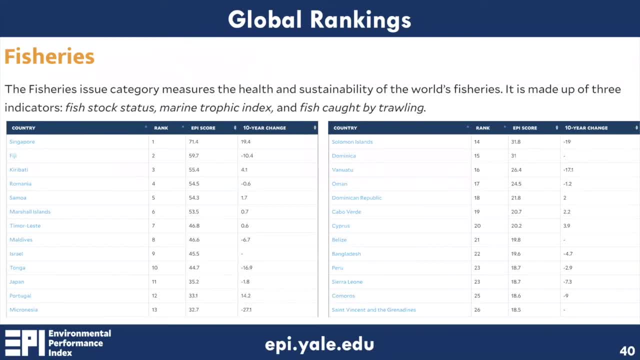 Okay, so this table summarizes the top performers overall in the fishing categories And you can see that Singapore is the top in the fisheries category and many small island nations are also top performers. There aren't many major countries that make it into the top 26 spots. 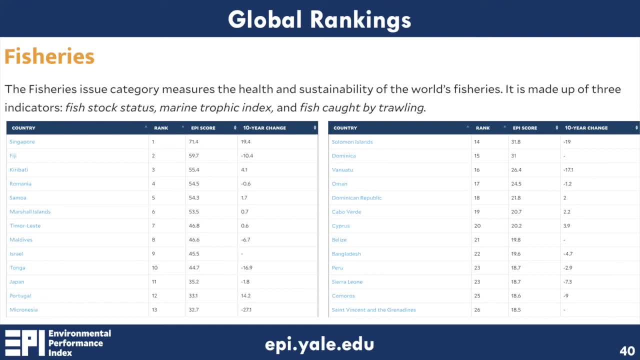 Canada, if you're interested, is 89, and the United States is 122.. So, again, we encourage you to go to our website and explore these rankings. Some of you may also be interested in the trends as well, the 10-year performance trends. 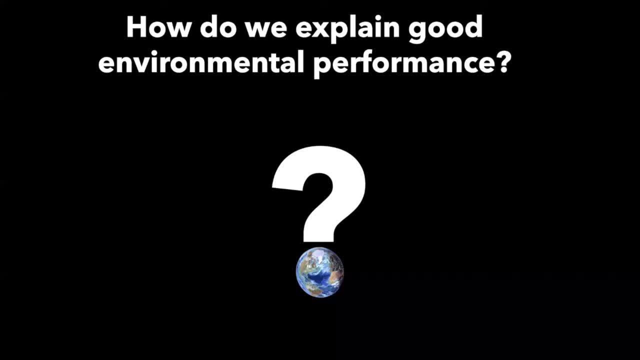 Okay, so in the last couple of slides of the presentation we've looked at some of the most important environmental performance trends in the world, But before I wrap up I wanted to just briefly touch on some analysis that I think asks a really important question. 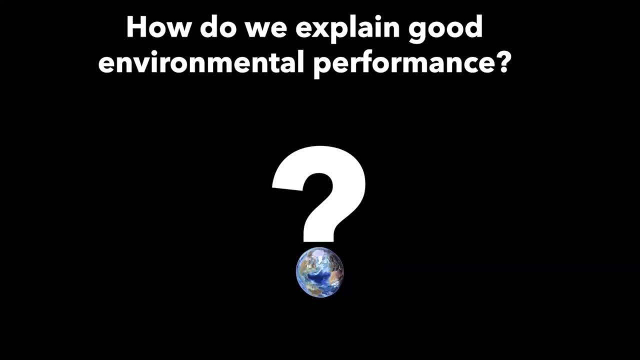 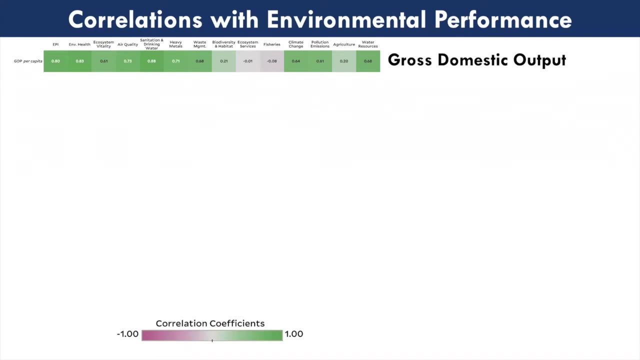 which is what drives good environmental performance. Why are some countries doing better than others, both globally and within peer groups? And we can't answer this precisely, but a really interesting analysis that my predecessor, Zach Wendling, and his team did was a study that showed that countries 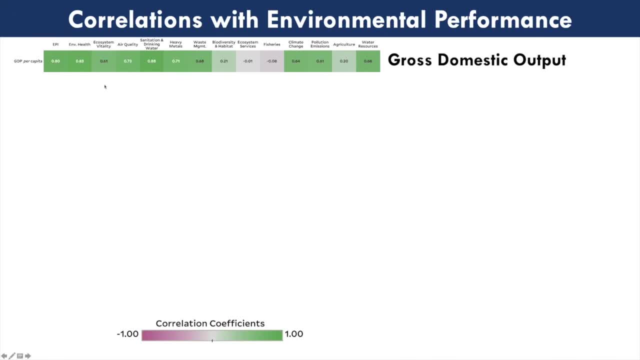 with a high GDP per capita generally have higher GDP performance between environmental performance index scores, as well as issue category scores and certain other governance, economic and regulatory variables. So just to go over a few highlights here, we're mainly interested in factors that correlate. 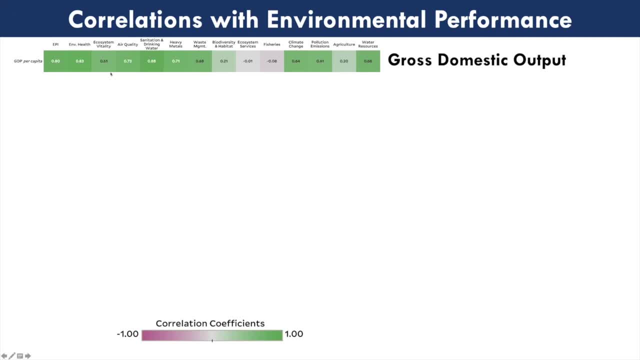 or don't correlate with good environmental performance. So countries with a higher GDP per capita generally have higher EPI scores as well as high scores between environmental performance index scores. So we also consider correlations with governance issues, So, for example, voice and accountability. 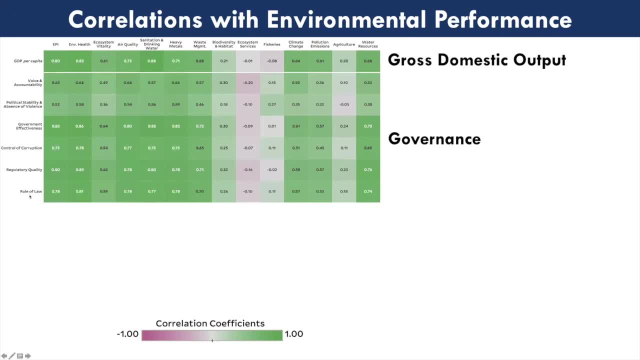 control of corruption. rule of law: We're suffering a bit in the rule of law category here in the United States recently And we can see a very strong correlation between things like government effectiveness and rule of law, et cetera, and environmental performance. 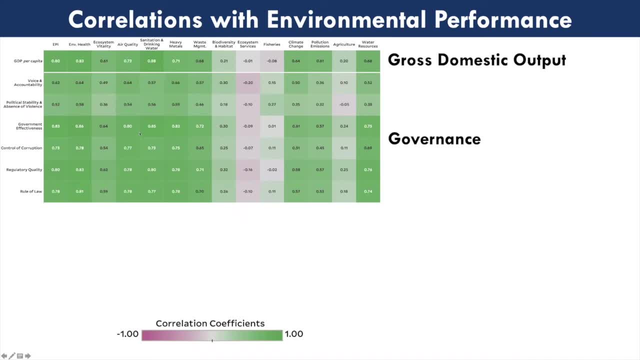 So the correlations between environmental performance and economic indicators are slightly weaker, but not terrible. Things like the contribution of services to GDP trade, so amount of exports in GDP- and manufacturing correlate less well than some of the governance indicators, And you might be surprised to see that manufacturing. 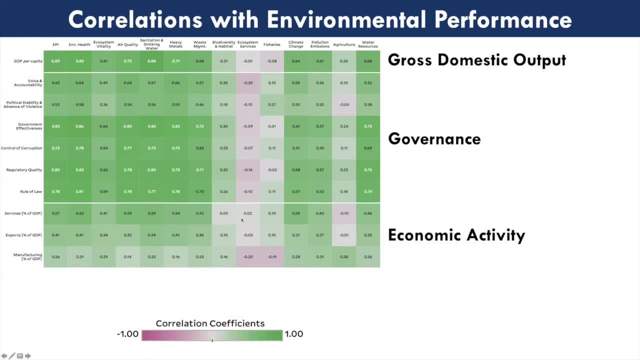 doesn't necessarily correlate with pollution- at least I was. So we do have two indicators here. Let me move on to the regulatory one, The regulatory aspect. Another surprising result of these analyses is that more and more stringent regulations don't always correlate with good environmental performance. 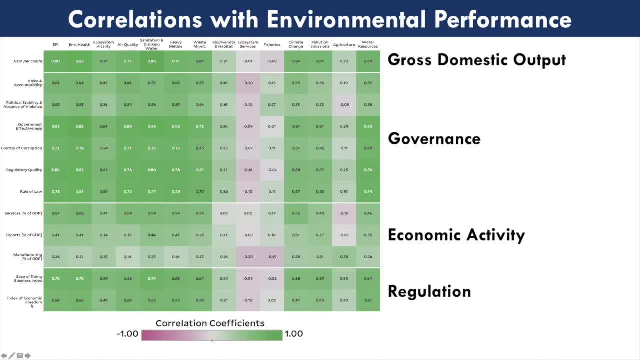 So the two indicators here- ease of doing business and index of economic freedom- both correlate moderately well with strong performance in most EPI issue categories. So I think the key takeaway here for this audience is that we really don't know what societal, governmental or economic factors 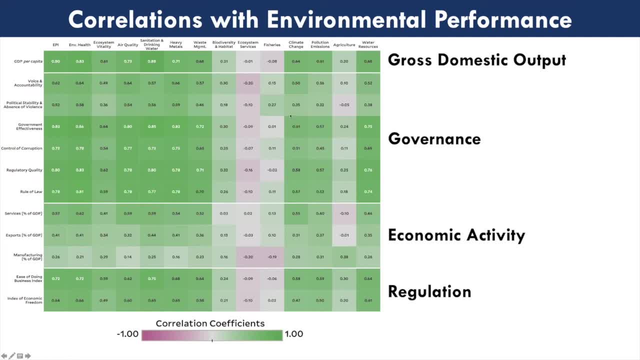 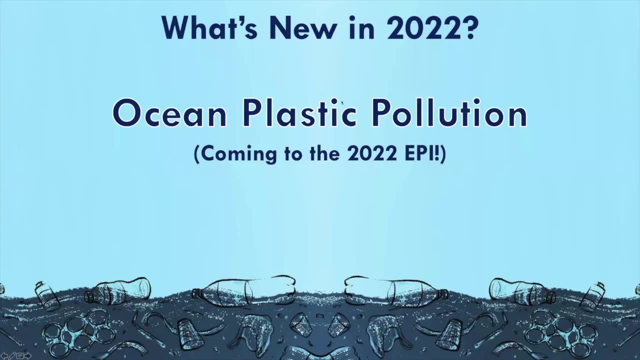 are correlated with sound fisheries practices. There's no correlations here, really. So we definitely need more work, more granular research, to determine what the explanations are of good fisheries practices. So the EPI is a continual work in progress And one thing that we hope to include. 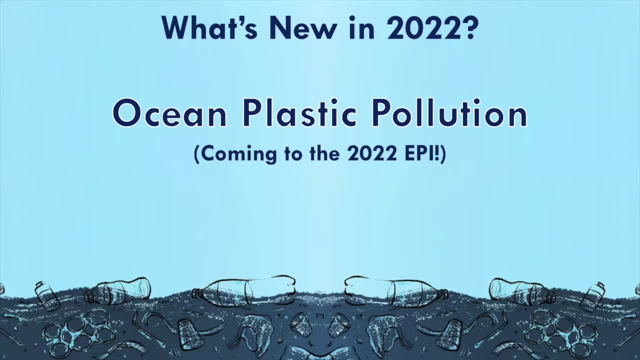 in our 2022 Environmental Performance Index is tracking ocean pollution, So specifically per capita emissions of ocean plastics, And there's been a flurry of research on this in recent years. If you know of any great data sets that are available out there. 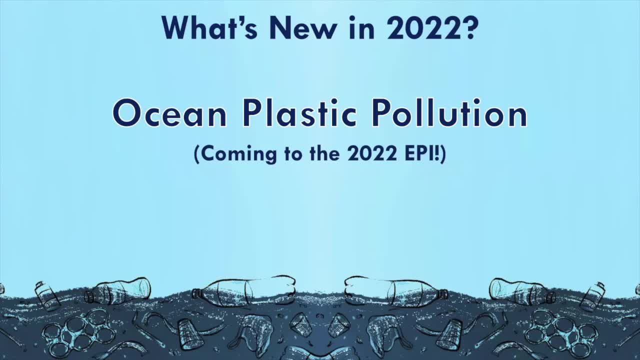 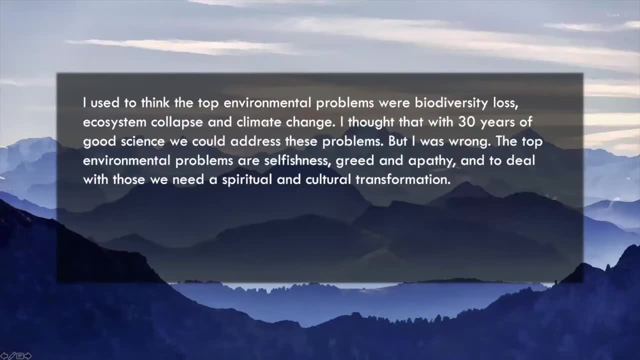 we'd be more than happy to follow up afterwards if you have ideas. We're aware of some kind of academically published data sets that we're currently tracking. Okay, So I'm going to quickly close off with a quote by Gus Speth. 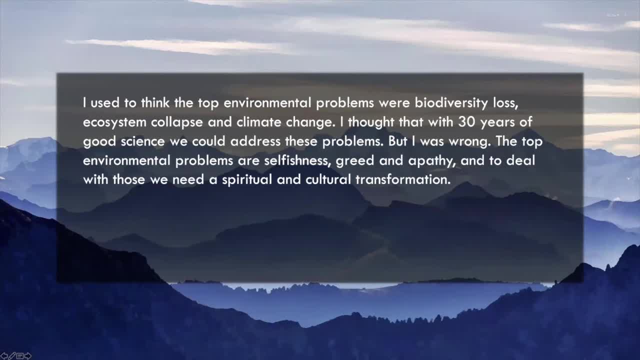 And I'll read it quickly for you, or we can read it together. I used to think that the top environmental problems were biodiversity loss, ecosystem collapse and climate change, And I thought that 30 years of good science with 30 years of good science. 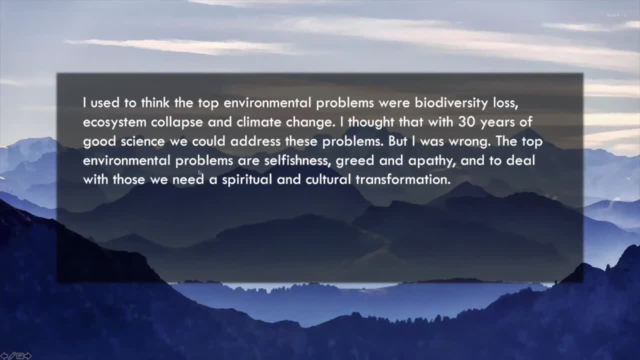 we could address these problems. But I was wrong. The top environmental problems are selfishness- fish in there, greed and apathy, And to deal with those we need a spiritual and cultural transformation. So he goes on to say that scientists don't really know how to deal with. 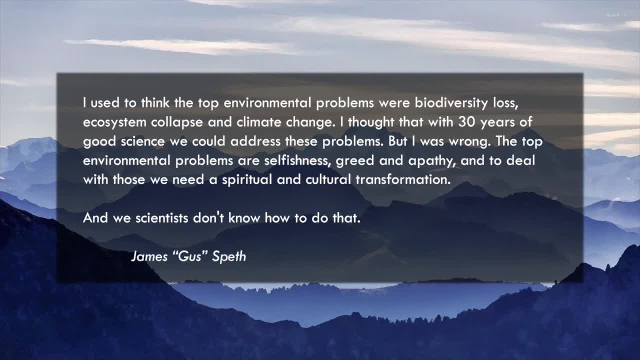 spiritual and cultural transformation. But I personally haven't given up yet on achieving good public understanding of environmental science and issues And I hope to have convinced you that analyses like the EPI that take complex, newly expensive data sets and distill them into a few key numbers and issues 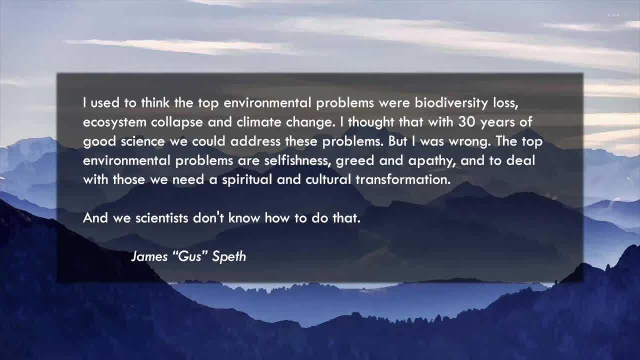 might be our best bet: to meet people where they are, at their level of understanding- not necessarily ours as experts- and achieve this needed goal, And so I'm excited to be here today to talk to you about how we can create a spiritual and cultural transformation. 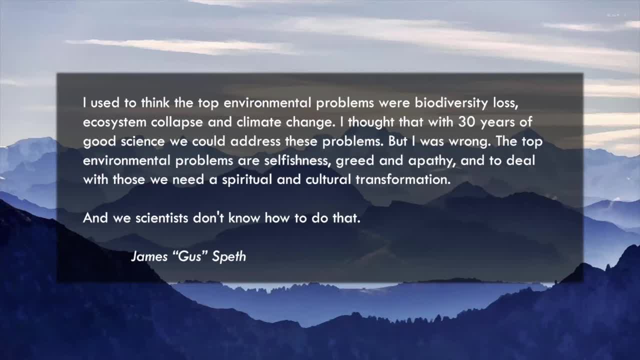 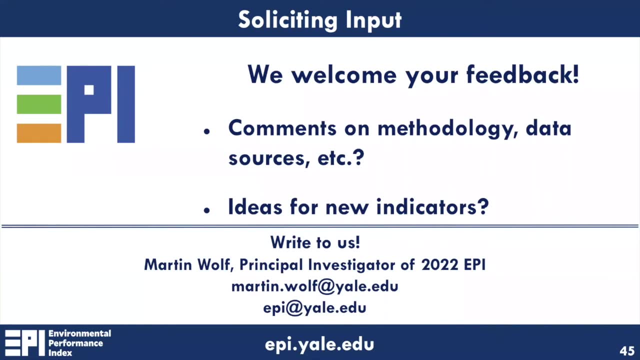 with data driven policy. In other words, data can be overwhelming, but it can also be empowering if it's used to present data correctly and comprehensively. So congratulations, you've made it through the presentation. So very grateful for having been given the chance. 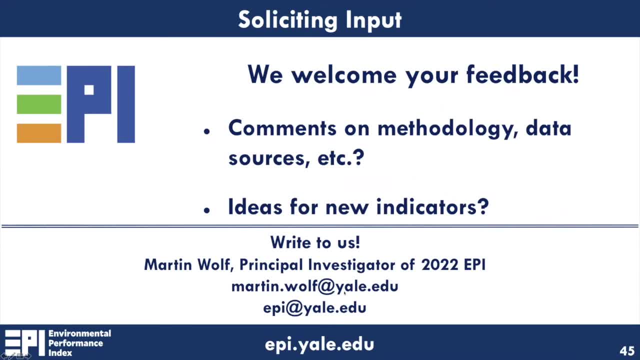 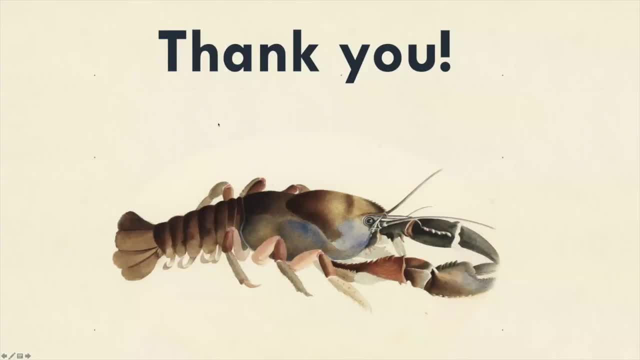 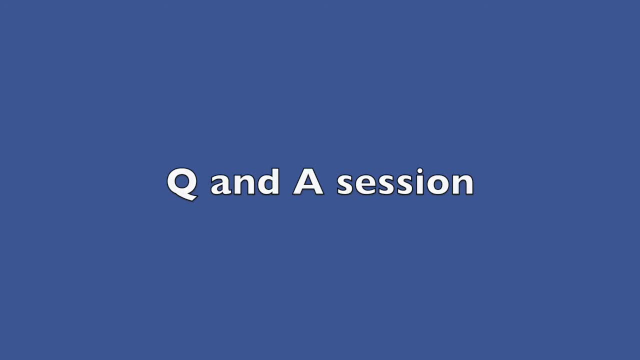 to come and present the EPI in our work to you. We welcome any thoughts you have now or later through our emails And we hope to hear and take any questions that you have, Thank you. Thank you, Martin, That was very. 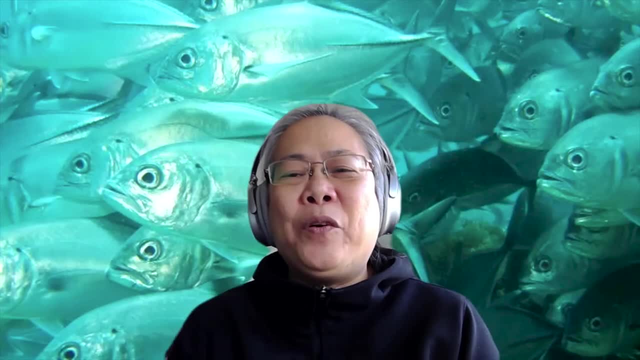 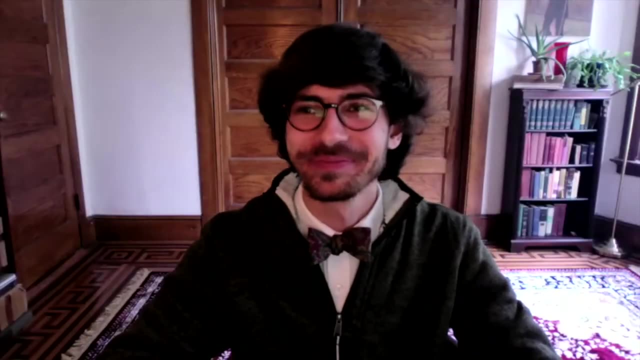 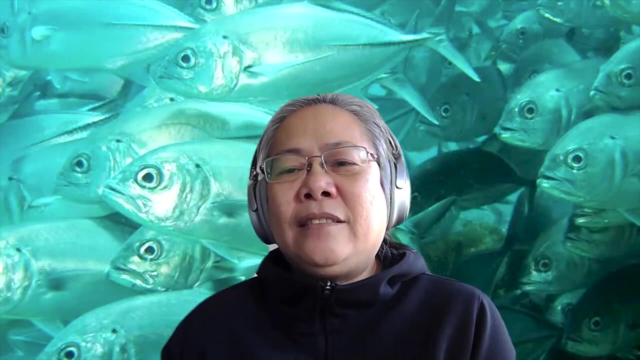 a very good presentation And now, for once, I understand what EPI is doing with the data that we provide. Yes, So my question is that your talk on marine protected areas right? You said 10% of the EEZ has to be protected. 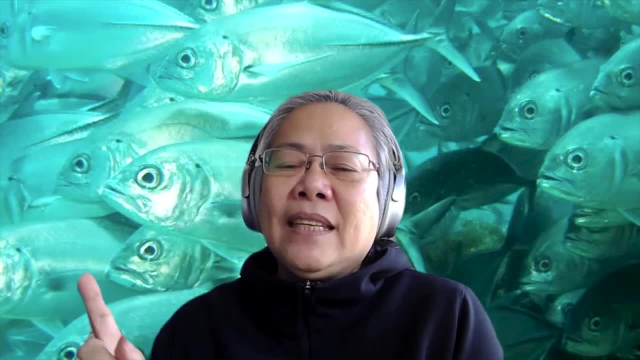 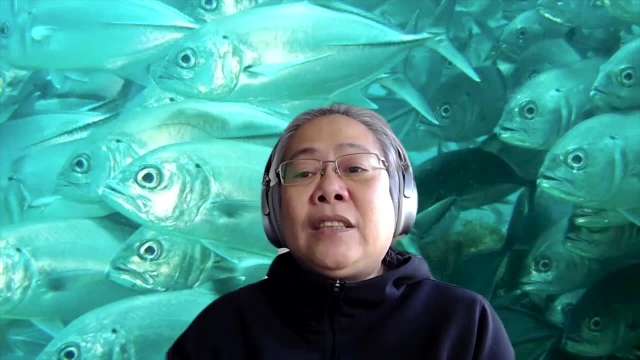 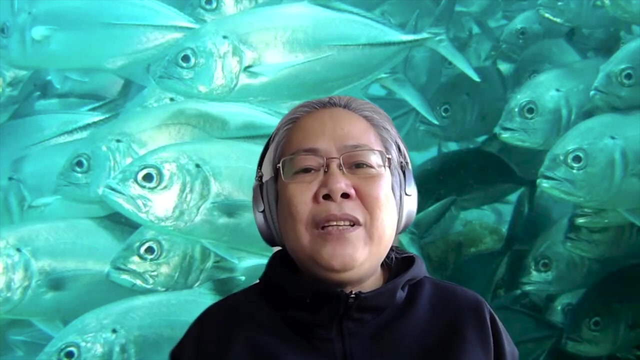 by all of these countries, right, But some of these countries have some of these MPAs have a mixture of protection levels, right. Some of them are no catch zones and some of them are mixed And most of them really are only an MPA on paper. 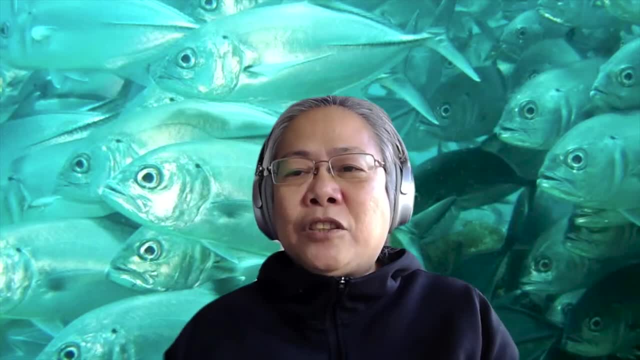 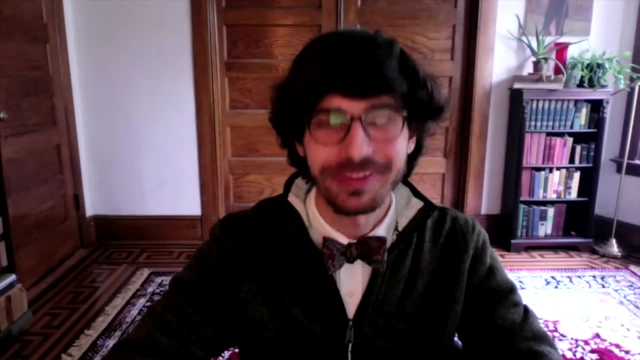 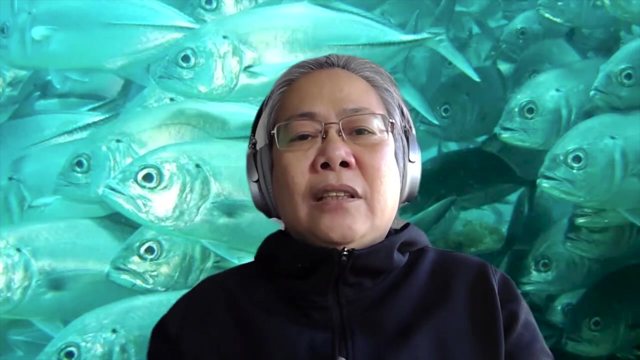 So there's no real protection on the ground, because protection means implementation and regulation, Right And enforcement And enforcement. So how is this protection enforcement regulation taken into consideration in your indicator? It's a great question And I guess the short answer is: 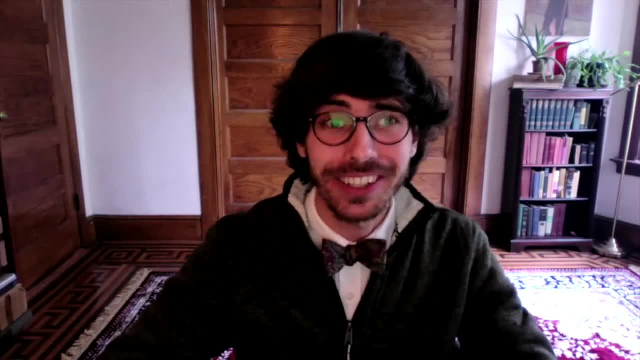 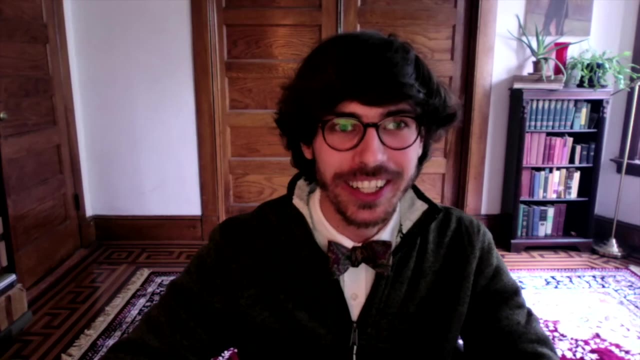 the enforcement level isn't really taken into account in our indicator. We use area and the area comes from the World Database on protected areas And you're absolutely right that maybe there's room for more granularity in different levels of marine protected areas- Certainly something we're willing to work with. 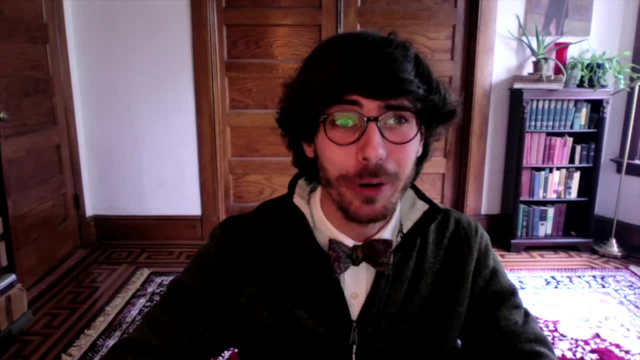 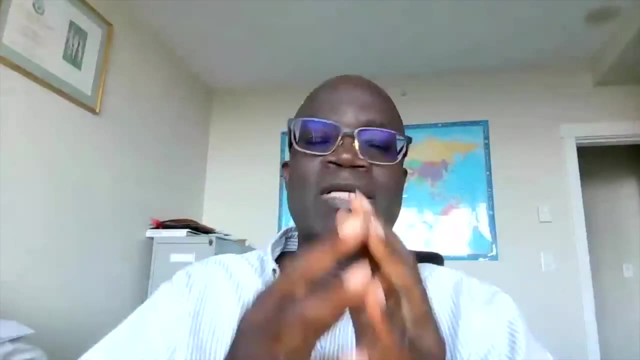 with you and your thoughts on, and developing a more, perhaps more robust indicator moving forward that also takes into account not just designation on paper, but designation in practice as well. Thank you, And my question is about the comparison of rich countries and poor countries, right? 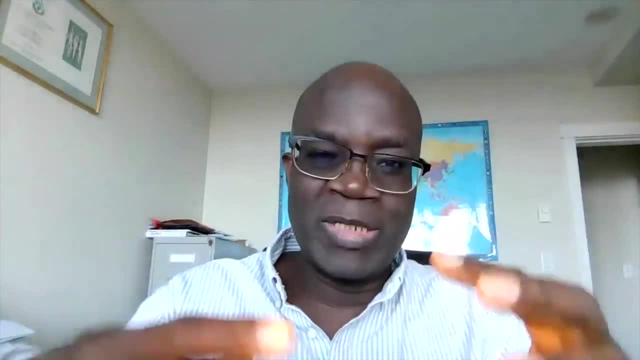 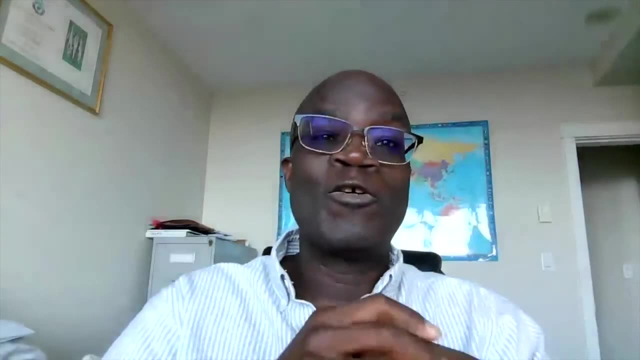 It's difficult to do that. It's difficult to do them like you said. So you went into peer countries, But maybe one way to do that is to normalize the scores against GDP, right? I mean, so you measure these countries from the holes from which they are standing, right? 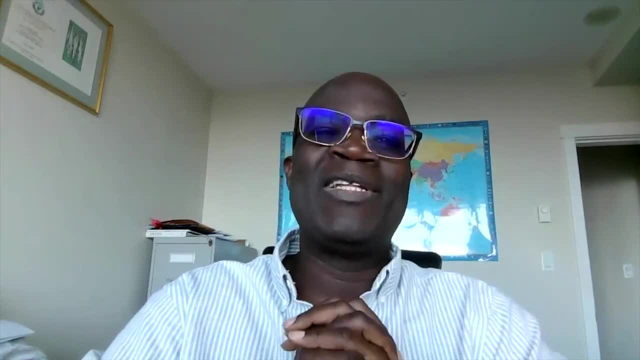 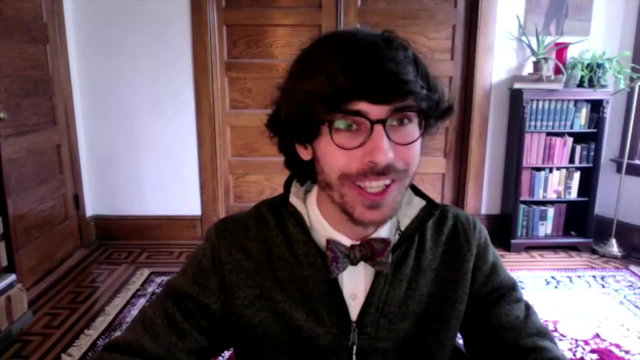 You know You might find out that actually Togo is the best, given the resources they have, rather than the US, where there may be too much waste. You know that? Yeah, absolutely, It's a really interesting idea for kind of like. 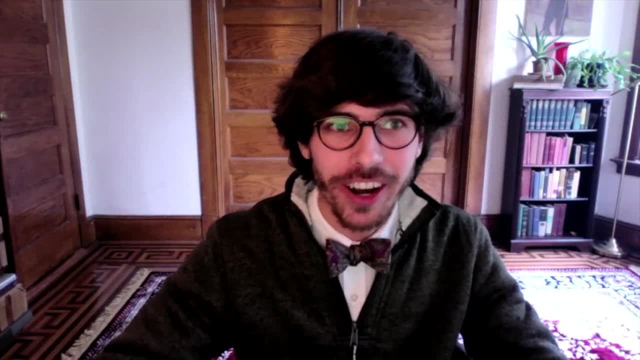 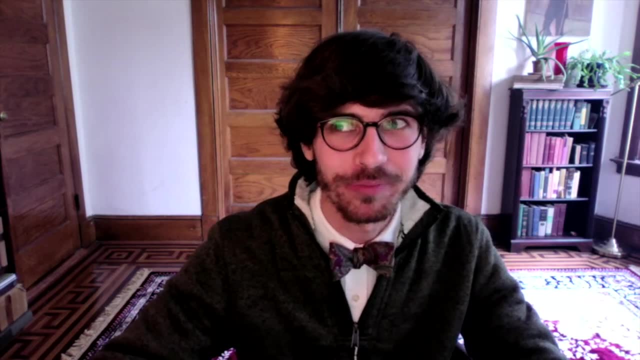 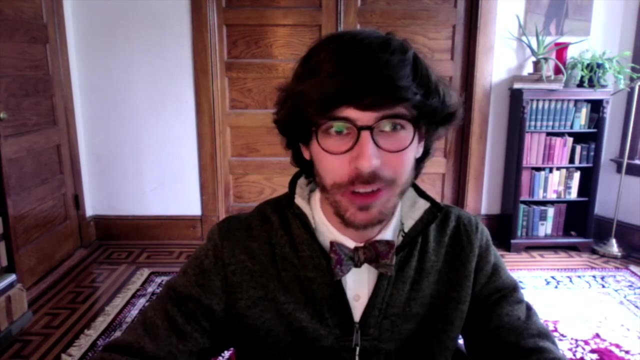 another level of analysis that we can do There are. we do normalize some things to make comparisons across countries more equitable, more fair. I guess you could say Another thing that, yeah, I really want to drive this message home because I think it's an important one. 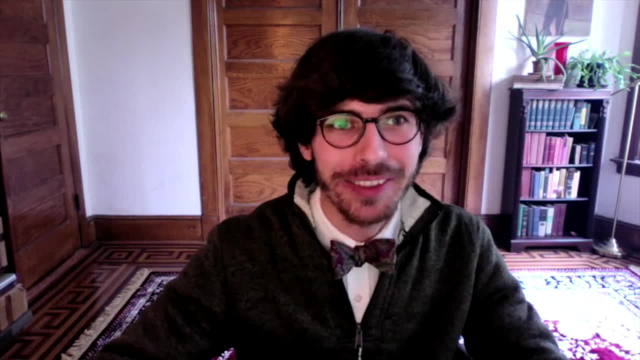 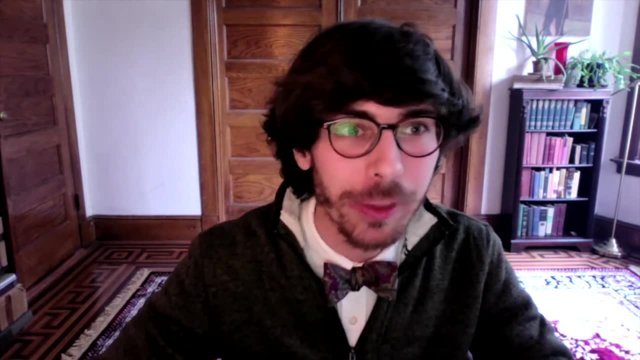 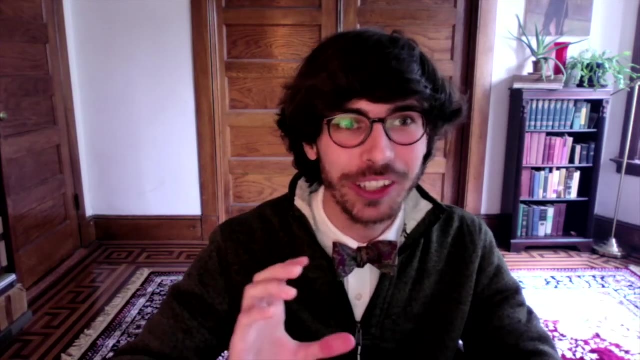 the one that you raised. The main takeaway of the API shouldn't be that you know the United States does better than a country like the Dominican Republic or something, But it's more fair to compare countries within their peer groups. Maybe peer groups can be established by GDP level. 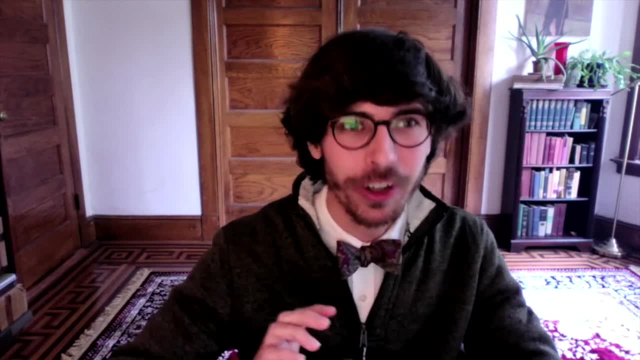 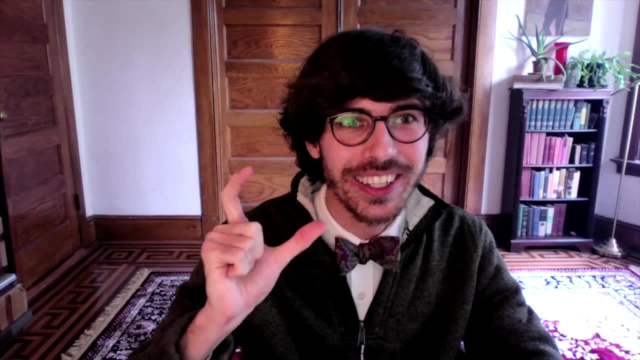 And what we see very interestingly, and I think very importantly, is that within countries that are very close in terms of their financial and political capital, there is a lot of variability. So I think that the main message of the API- the best use of the API results- is: 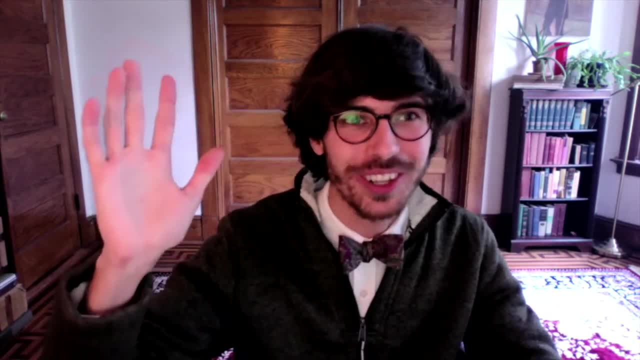 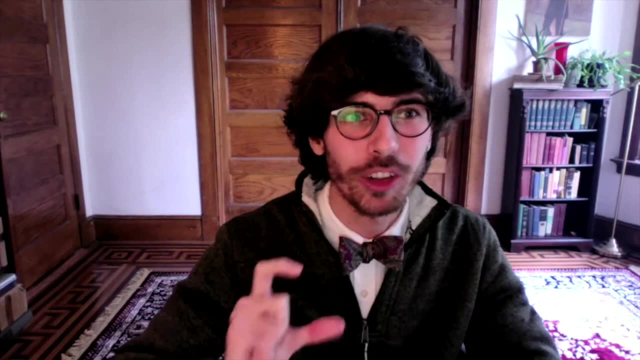 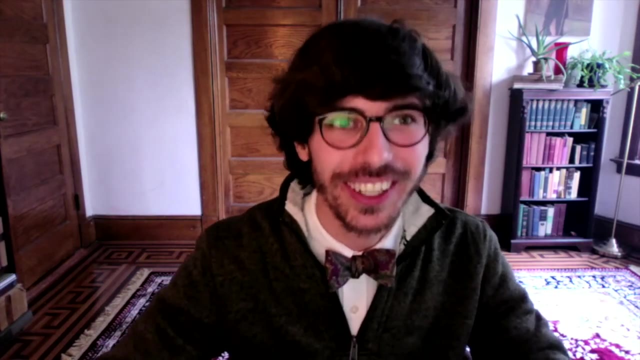 compare yourself to your peers, Don't you know? we're not asking you to compare yourself to the top performing countries. Compare yourself to your peers and work together, collaborate to see which policies can be distributed better. But your point about, yeah, normalizing for other. 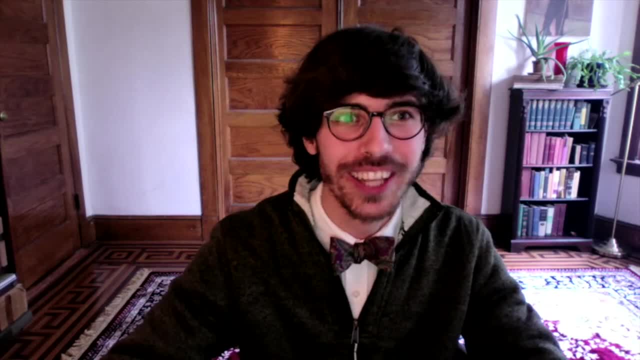 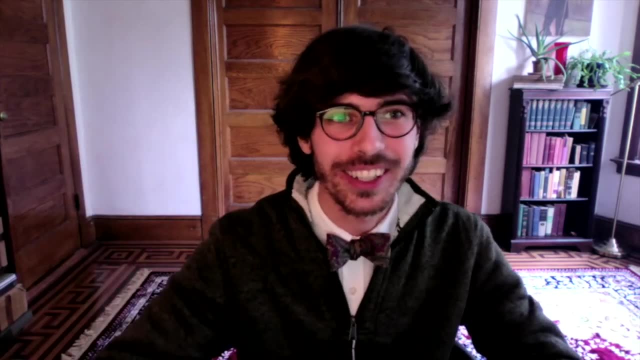 you know, economic variables is a great one And we're kind of moving towards that with this recent analysis that I was describing at the end, kind of doing correlations with economics, variables and GDP. So, thank you, Thank you, Rishi, Thank you. 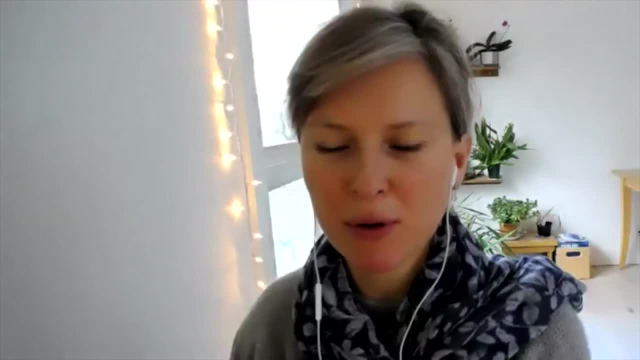 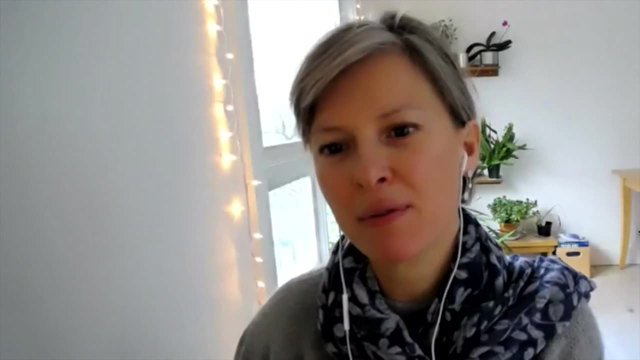 So Simon said that he'd be happy for one of the facilitators to ask one of his questions. I wonder why the correlations are so weak for fisheries compared to many of the other indices and whether you have some initial thoughts or ideas in that regard. 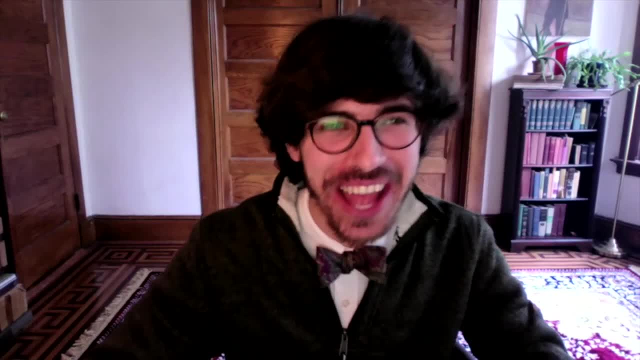 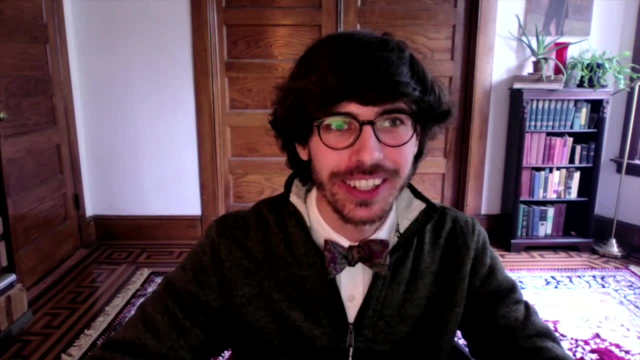 I wonder too, Simon. I'm sorry, Part of it could be due to you know we question how accurate the data is. You know some of those. I think different countries have different accuracies in terms of the data. I see Deng nodding her head. 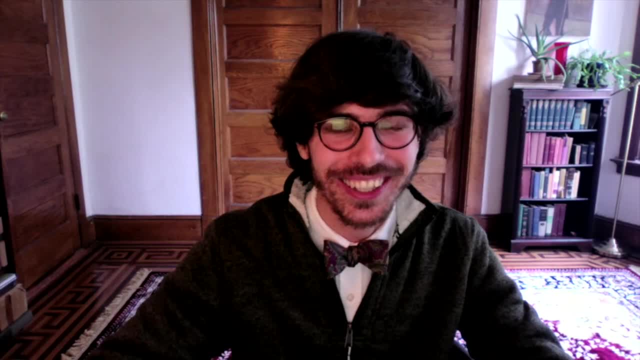 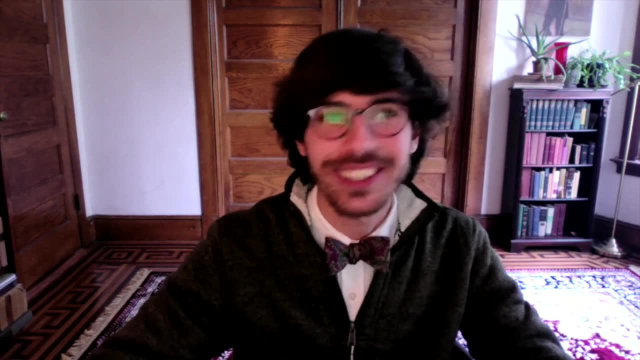 You know we always. you know it's not to say that see around us is compiling inaccurate data, but we do the best we can with the methods that we have now, right, So maybe as data sets become more robust and with new, you know. 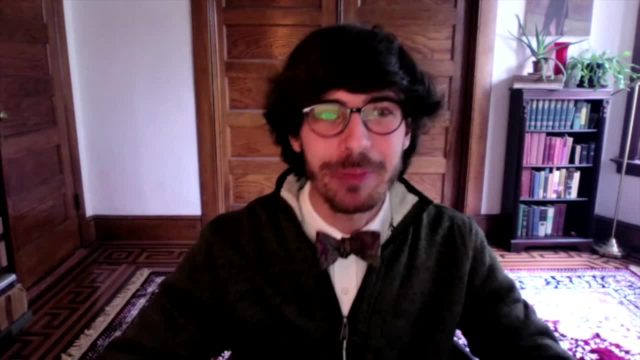 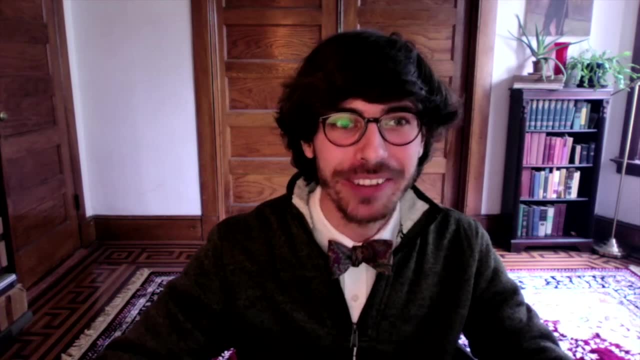 maybe remote sensing technologies, kind of verifying data, maybe we'll see correlations become better. But yeah, if you have any ideas as to things we could explore about why fisheries don't seem to be correlated while other issues are correlated, I'd be happy to talk more. 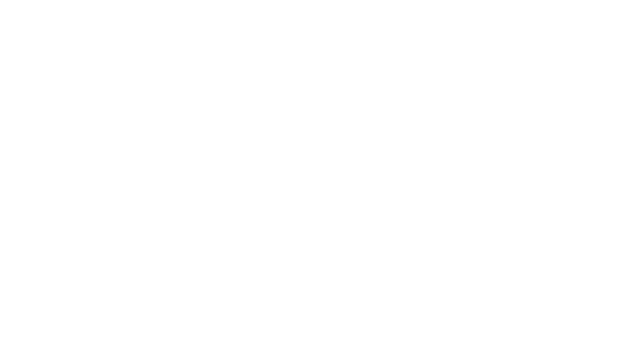 about them afterwards. Hello and thank you for the great presentation. I was just wondering: is ecosystem loss treated the same across a variety of land conversion types? So, for example, is tree cover conversion to urban or agricultural land ranked as a greater impact on EPI? 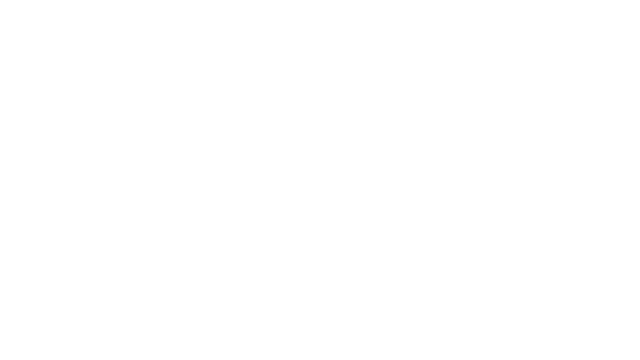 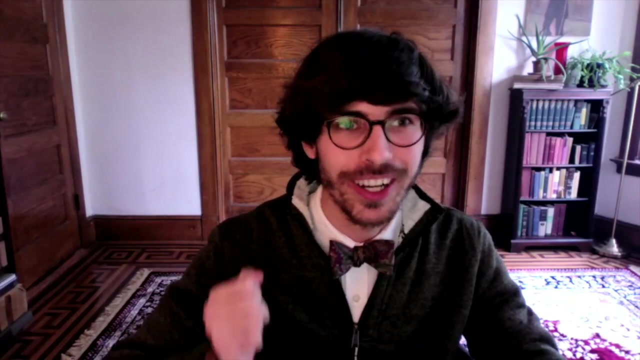 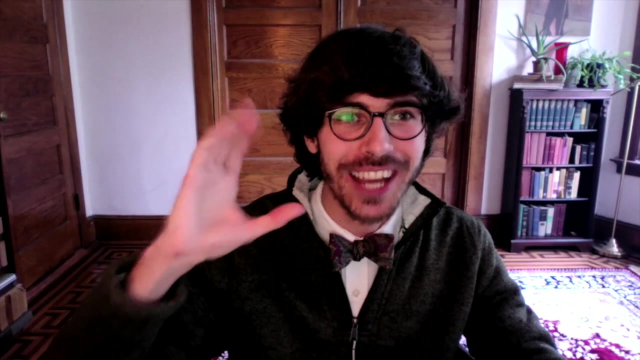 than tree cover loss with deforestation? That's a great question. The answer is no. Specifically how we check ecosystem loss? right now we have tree cover loss, wetland loss and grassland loss. We compare the amount of area loss to its baseline. 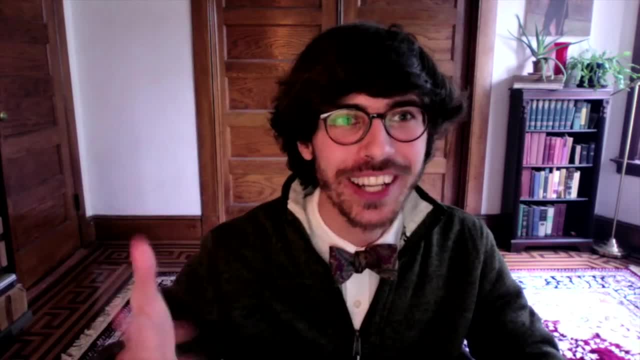 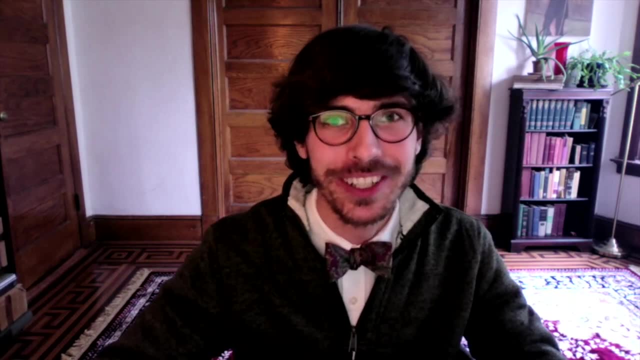 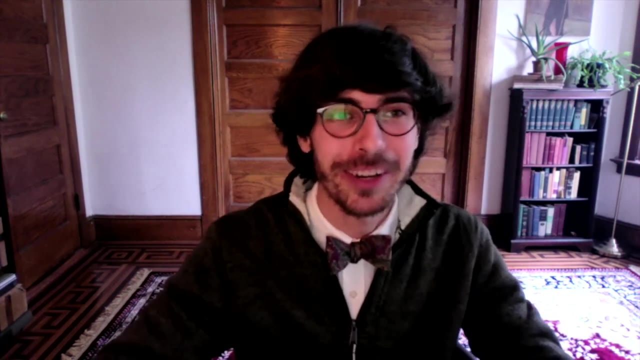 which is about 20 years ago, when good satellite, you know robust satellite data was being compiled. But if a forest is converted to agricultural field, versus forest converted to, you know, a suburb or really an urban environment, we're agnostic to the conversion. 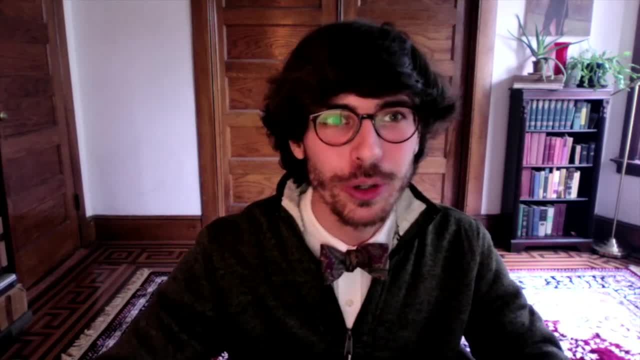 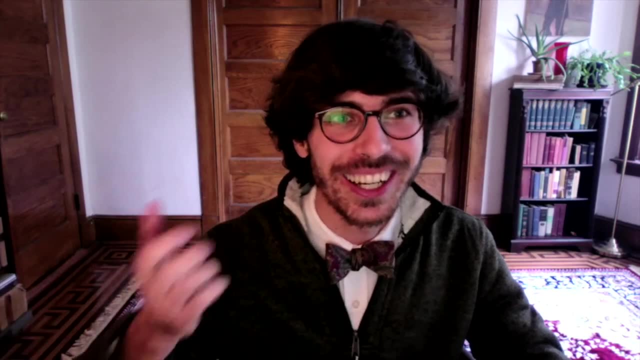 Where it does come into play is the CO2 emitted from land cover change. So conversion, converting a forest to an agricultural field has a different emission factor than converting it to something else. right, So we do consider it there, but just in terms. 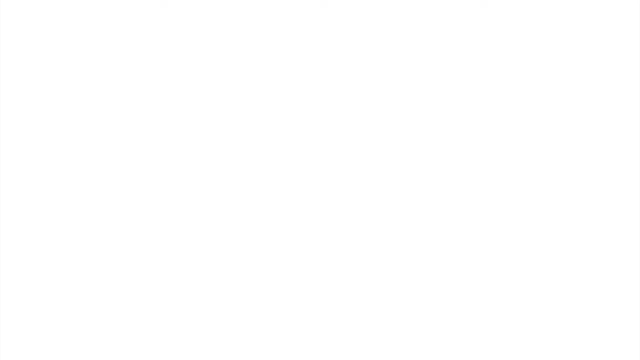 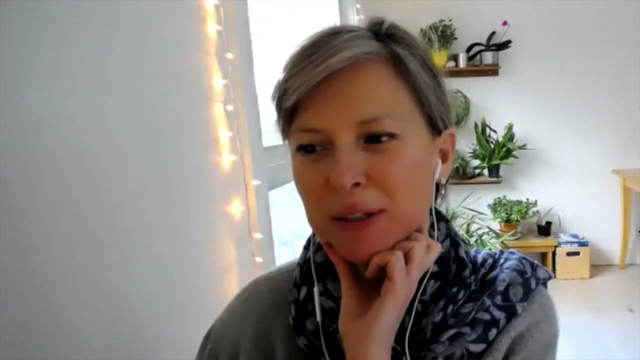 of actual ecosystem extent. we're agnostic to where it ends up. We only care about you know what's being lost. So I will take the liberty- and I hope this is all right with Simon- to ask one of his other questions. 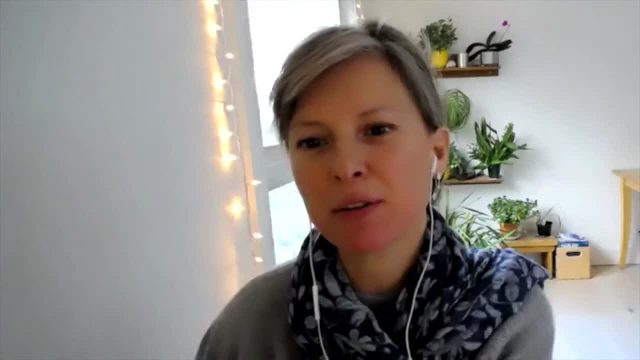 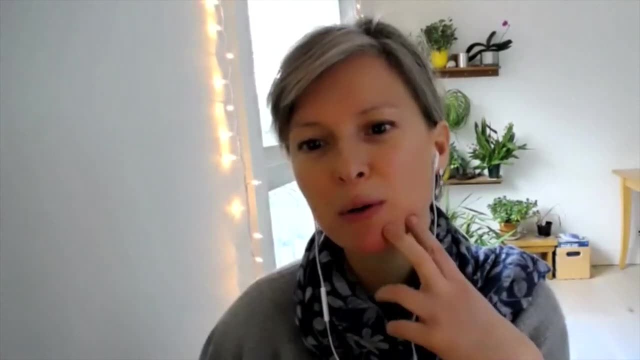 which was at the beginning. He was wondering. he saw that you know, in the slide that you had, where you outlined some of the pollutants, for instance, that heavy metals were included, And so whether that was like, whether that was a conscious choice. 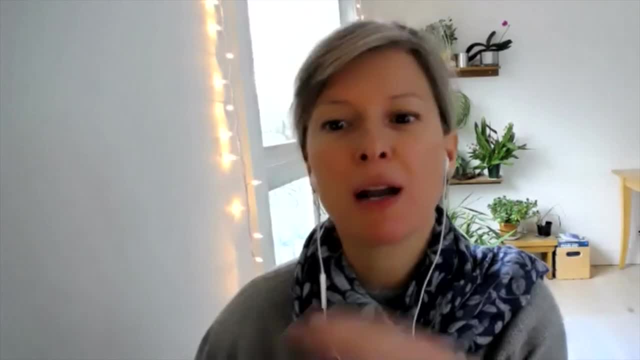 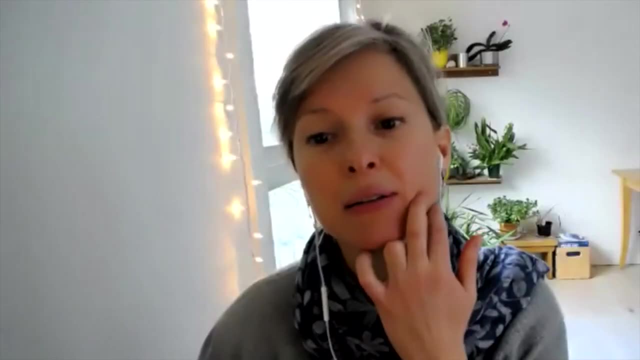 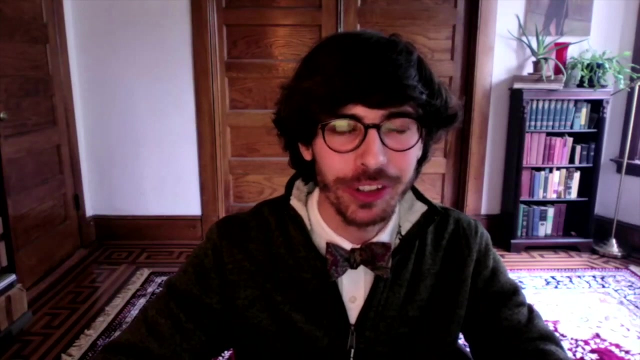 and did not include, for instance, persistent organic pollutants, or at least these were not included in the slides. If that was a conscious choice, why was that choice made? We get our pollutant exposure data from the Institute of Health Metrics and Evaluation, Global Burden. 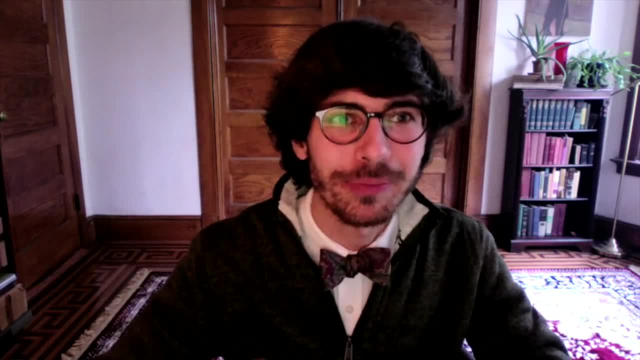 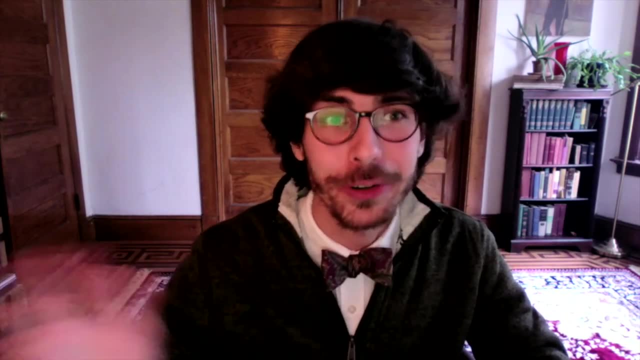 of Disease Analysis, And so that's where, for example, exposure to lead came from. I included it in the atmosphere slide, but it really takes into account morbidity and mortality from all sources of lead, be it paints or water or soils. 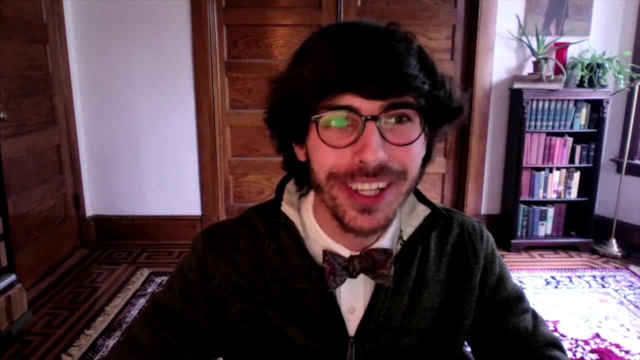 In terms of persistent organic pollutants. that's a great example of an important indicator, an important issue that we don't have, or at least don't know of good global data sets for. We might have good global data sets for, maybe, developed countries or maybe especially the European Union. 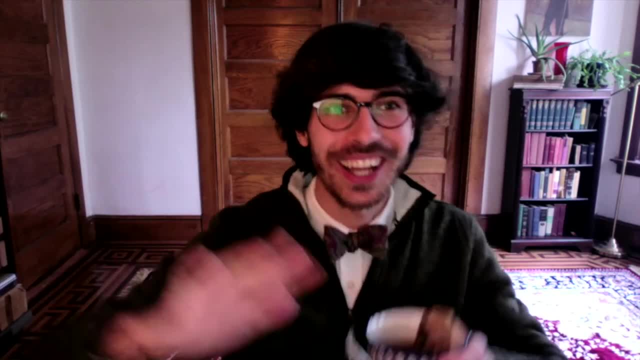 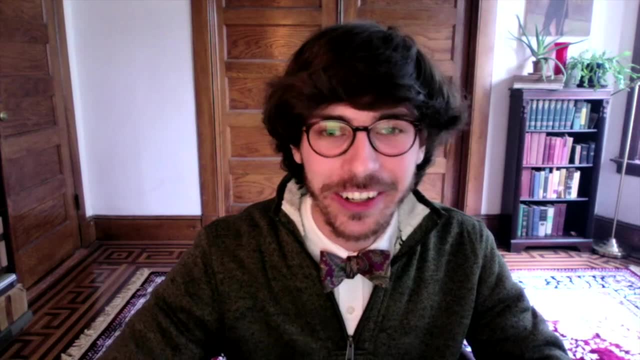 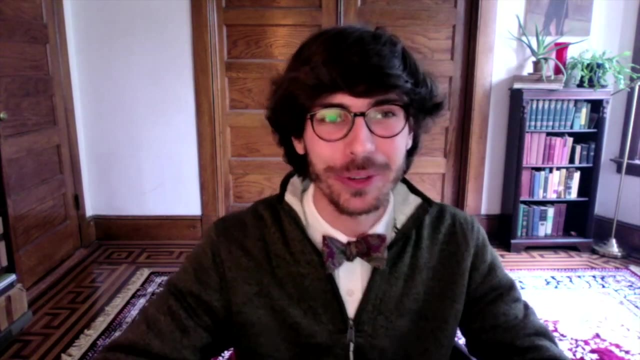 but we don't have good enough information on a global scale in order to include things like persistent organic pollutants in our API If we're unaware. if you know of a good data set on persistent organic pollutants or anything that you don't think we're aware of. 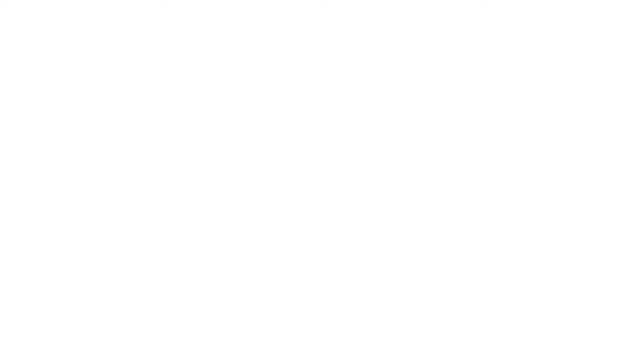 please let us know. We'll be happy to include it. I was just curious if you had any consideration into using longer-term baselines. so, rather than 20 years back, thinking about hundreds of years, thousands of years back, using paleoarchaeological. 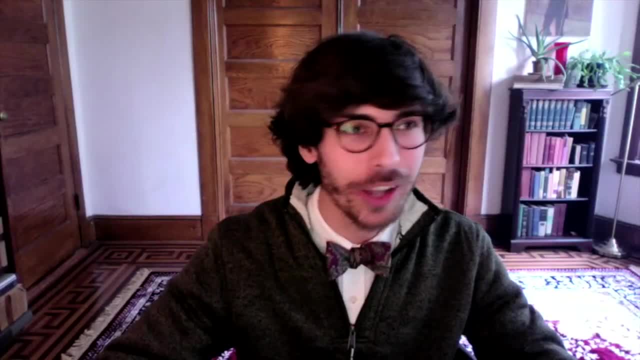 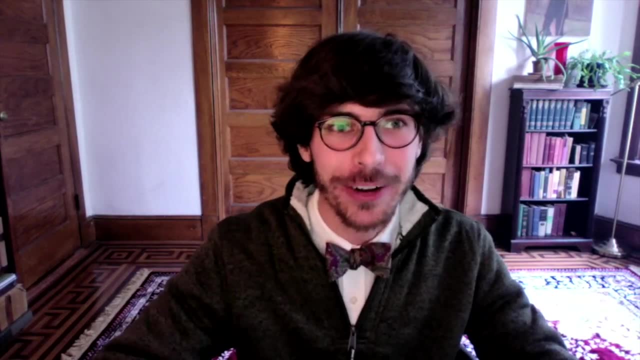 and paleoecological data. Oh, it's such a good question, Something that we're considering doing. that for particularly are greenhouse gas emissions. So right now, if let's- I'm laughing when I say this- but let's decide the United States.